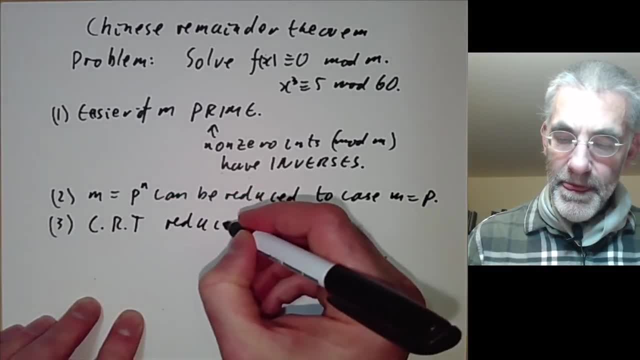 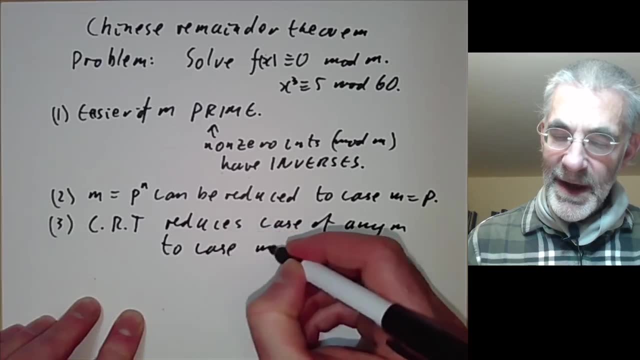 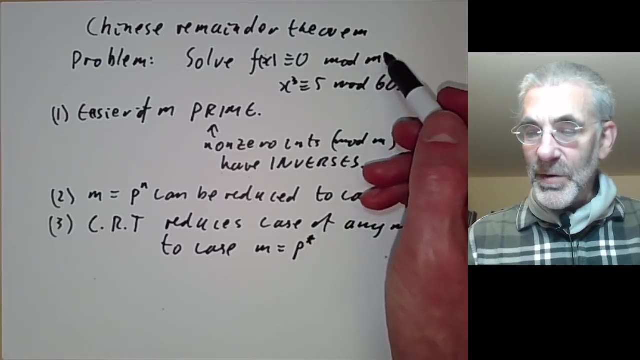 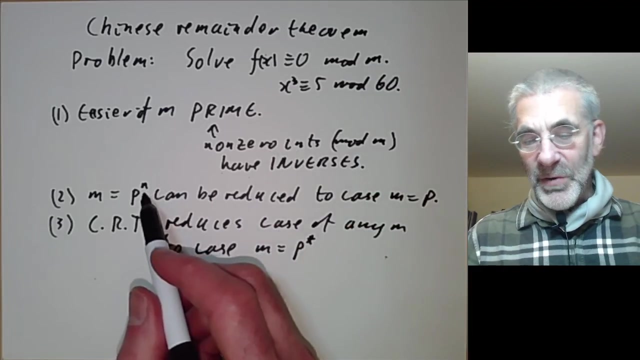 remainder theorem reduces the case of any m to the case when m is a prime power. so so the general technique for solving a congruence modulo some number, is we first going to use the Chinese remainder theme to reduce the case of prime powers? then we reduce the case of prime powers to primes, using things like Hensel's. 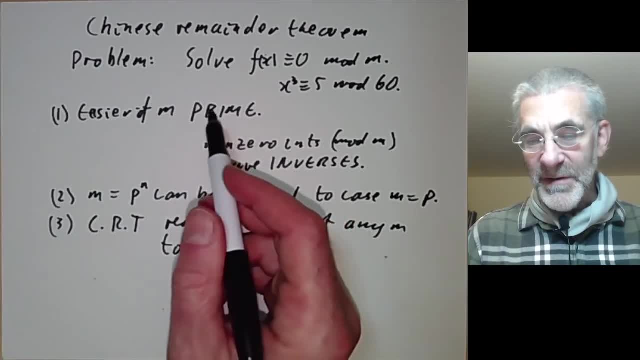 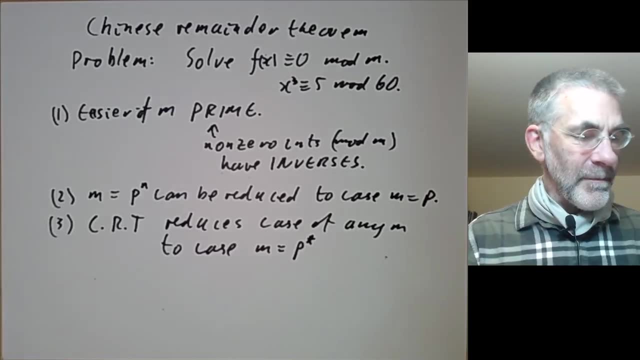 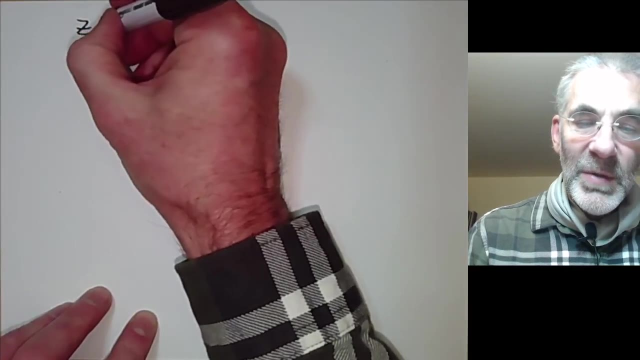 lemma. and then we solve for the case when m is prime by using the fact that the integers modulo a prime are particularly well behaved. so before going on, I just want to introduce some standard notation. so we generally write Z modulo MZ for the integers modulo M. so it would: 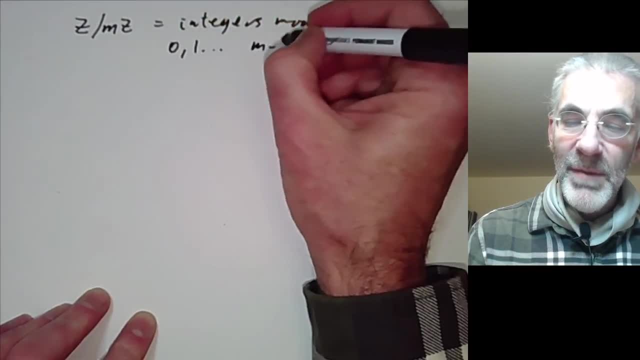 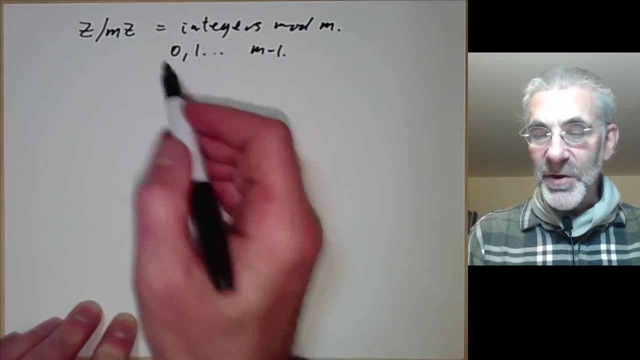 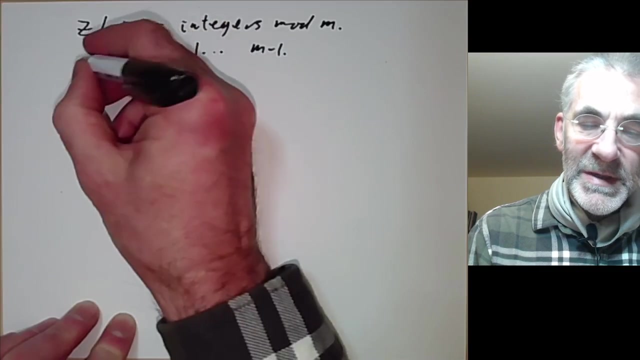 be the integers represented by 0, 1 up to M minus 1, and this is a ring, meaning you can do addition and multiplication on these, and it satisfies many of the usual properties. we're also going to use the notation Z over MZ times to be the 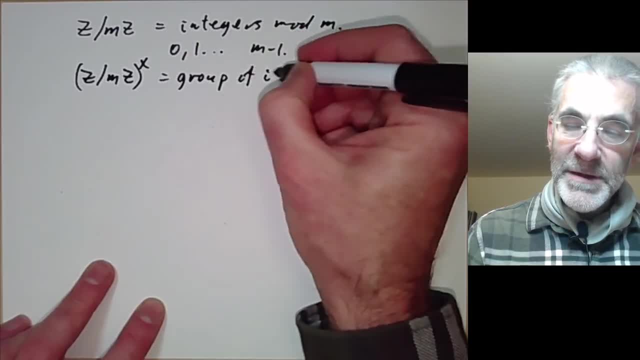 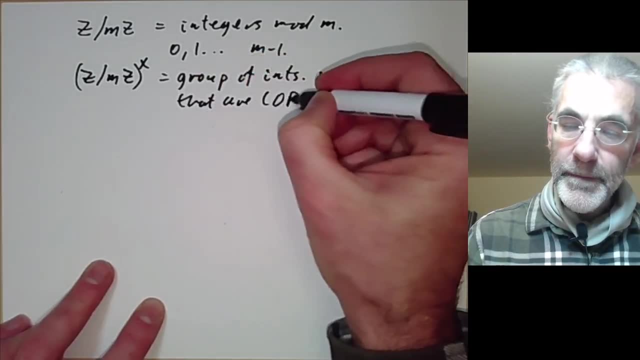 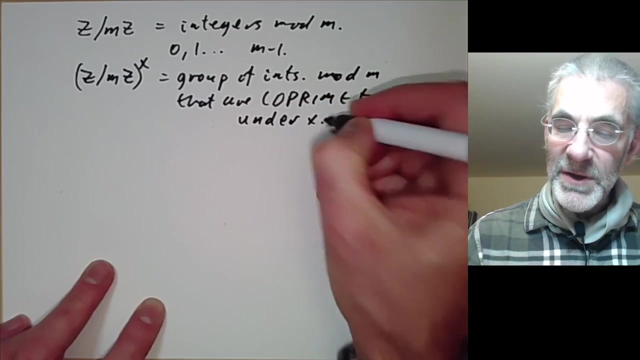 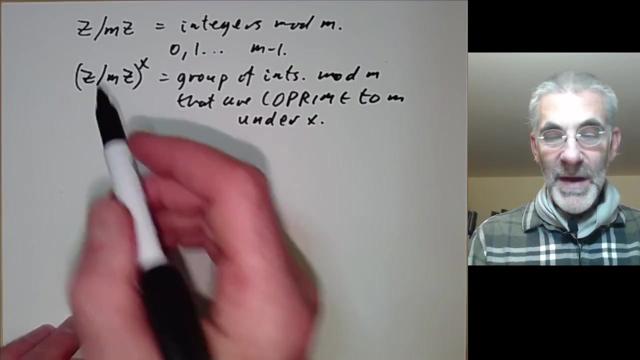 group of integers modulo M that are co-prime to M under multiplication, and we're thinking of them as being a group under multiplication. so you remember, we check that the integers co-prime to M were closed under multiplication and have inverses and so on, and it turns out to be one thing you need to use a lot of. 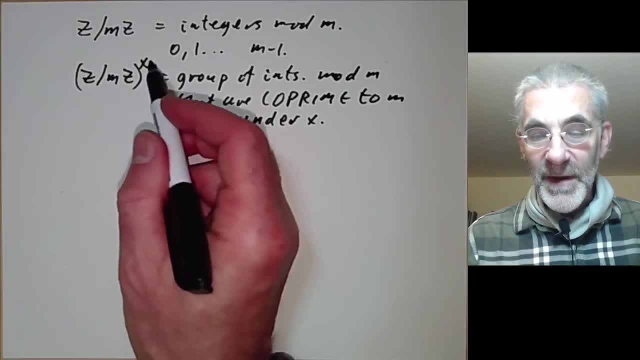 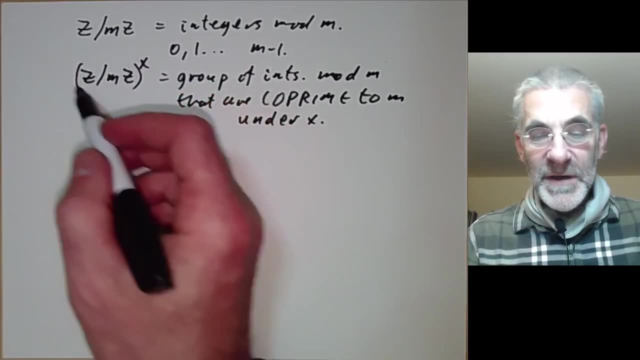 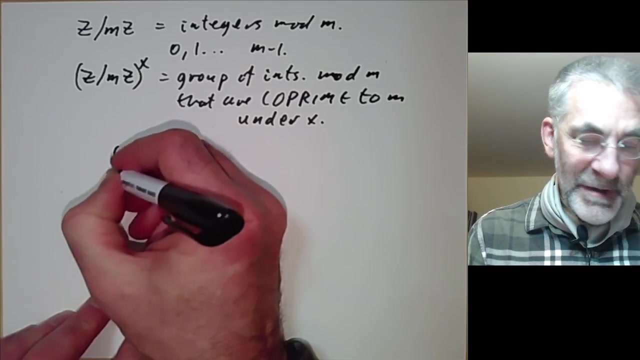 your memory to get the right answer to that question. so the last thing we're going to do is to look at the structure of this group and what they do, and how does this group behave? one major application of the Chinese remainder theorem will be to try and understand the structure of this group, as we'll see. 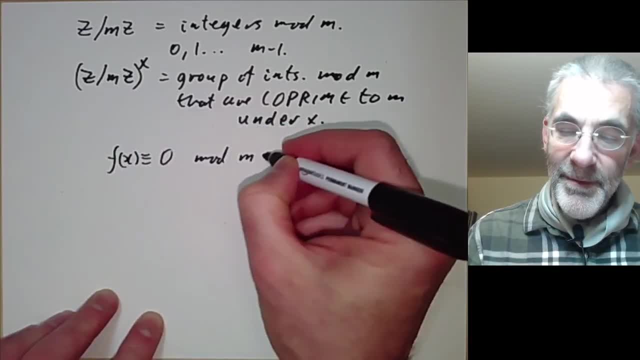 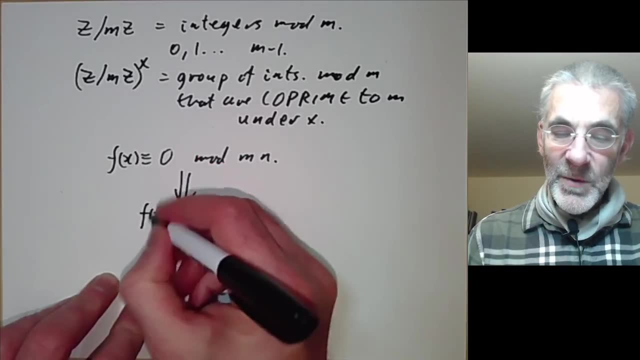 later. suppose we want to solve the equation f of x is congruent to zero modulo MN. well, suppose we found a solution. then we can certainly solve. the equation f of x is congruent to zero modulo MN. then we can certainly solve this. the equation f of x is congruent to zero modulo MN. 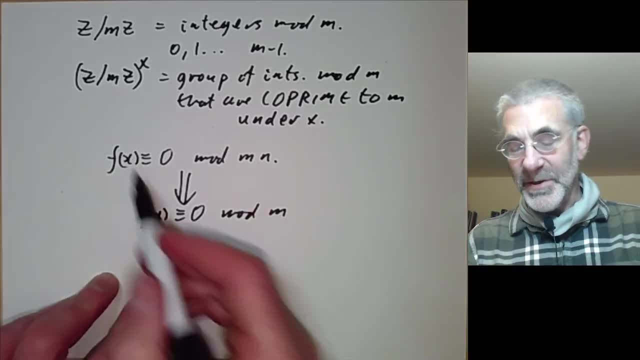 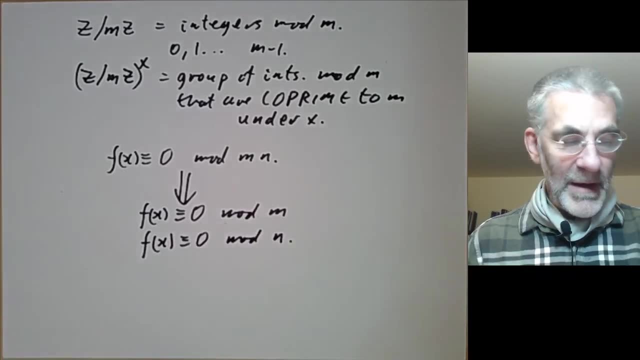 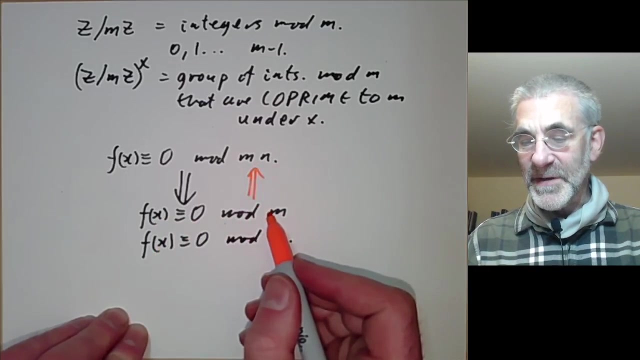 to zero modulo m, because we can just use the same value of x and we can also solve the equation f of x is equivalent to zero modulo n, and the question is: can we go back the other way? so suppose we can solve this equation for some x and this equation for some possibly different x. can we then solve? 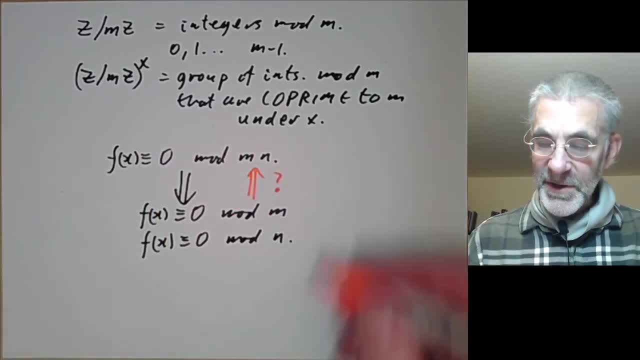 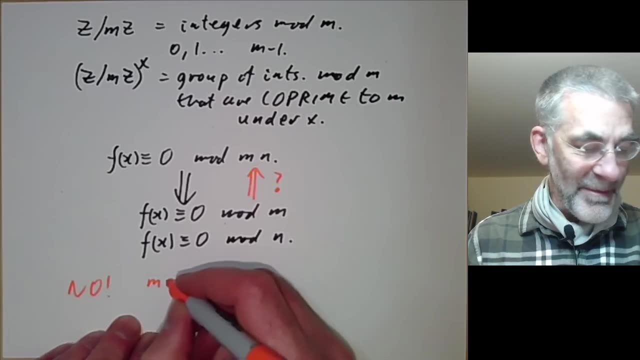 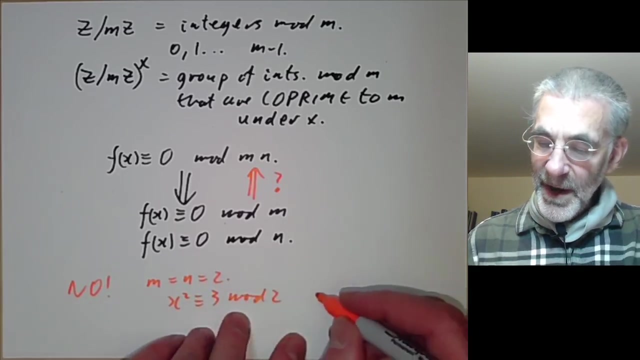 this equation. let's put a question mark and the answer is no. we can't generally go back, and it's very easy to see cases when you can't. we can just take m equals n equals 2, say, and then we can solve x squared is congruent to 3 modulo 2 and we can solve x squared is congruent to 3. 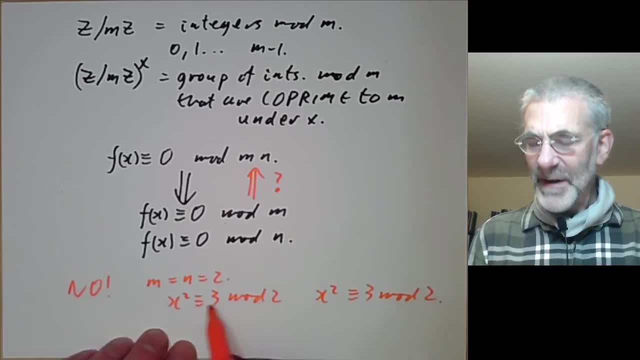 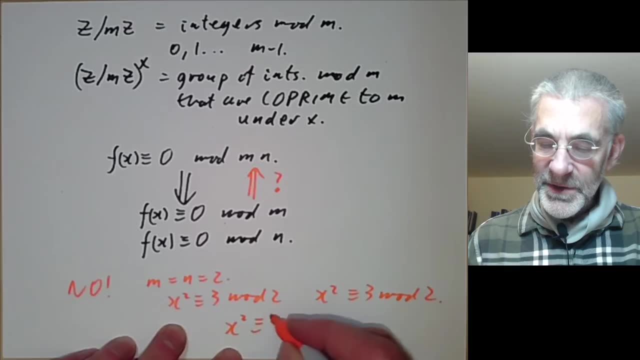 modulo 2 and it looks exactly like this equation. in fact, it is exactly this equation. since m is equal to n, we can take the same equation. but if we try and solve x squared is congruent to 3 modulo 2 times 2, we're stuck. this, this equation, has no solution. 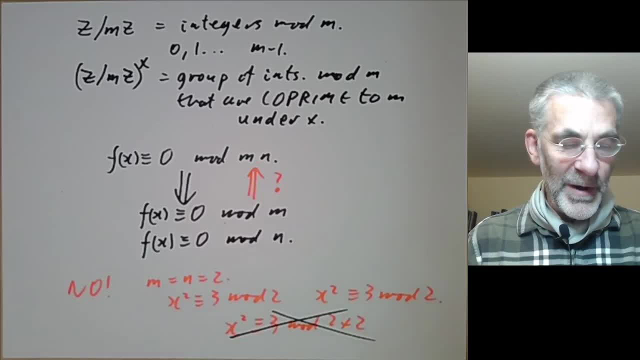 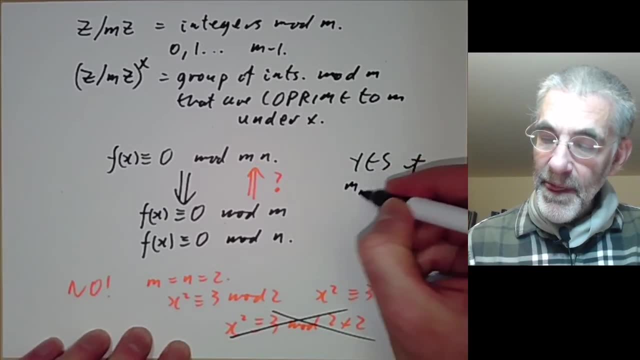 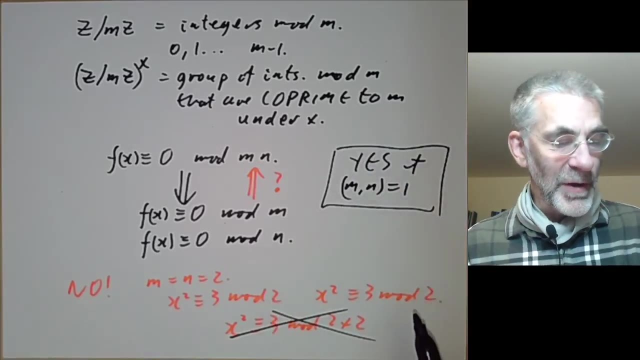 so we can't always go back the other way, um, however, we can if m and n are co-prime. so you see, the problem in this case is that two and two are not co-prime, and there are two ways of doing this or seeing this. so there's first of all the 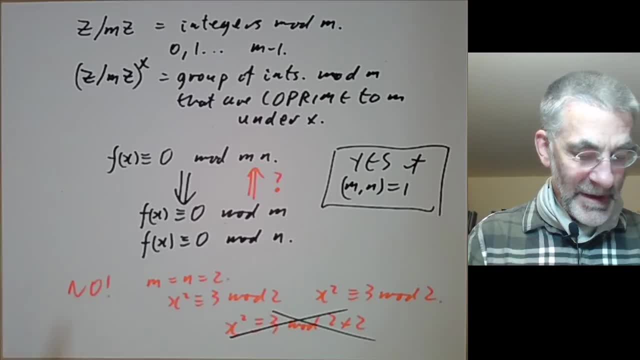 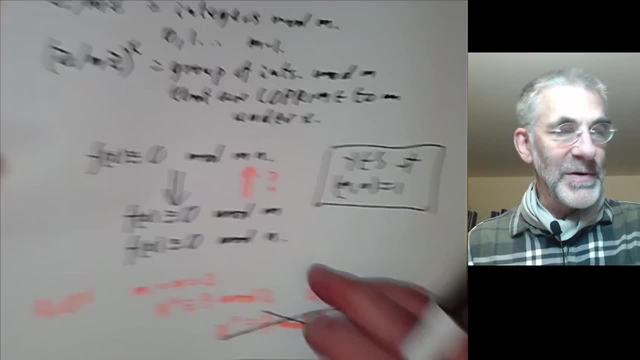 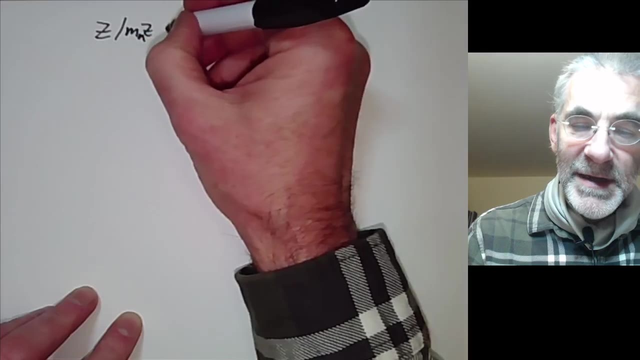 co-prime, a sort of abstract method, and then there's a sort of computational method. So I'll first do the abstract method, which what we do is: we look at z modulo m n z and we map it to z modulo m z. 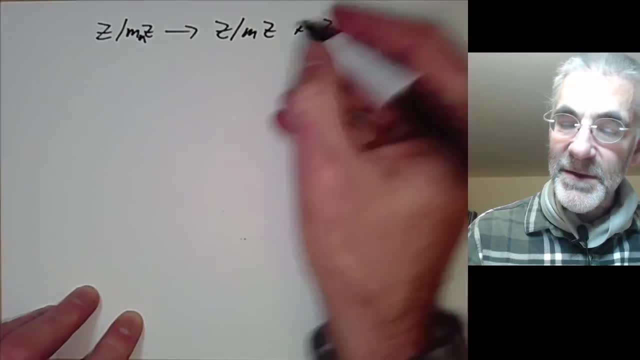 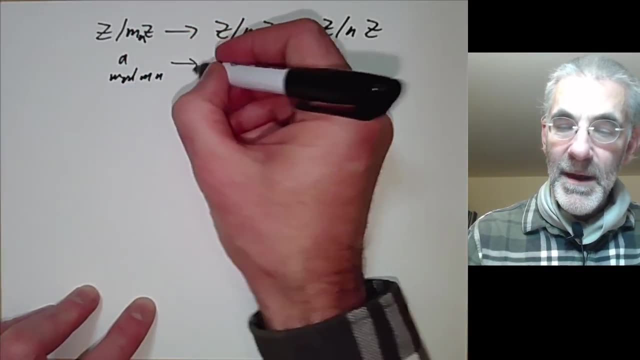 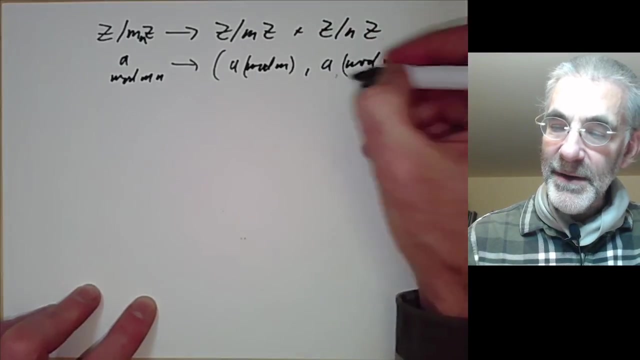 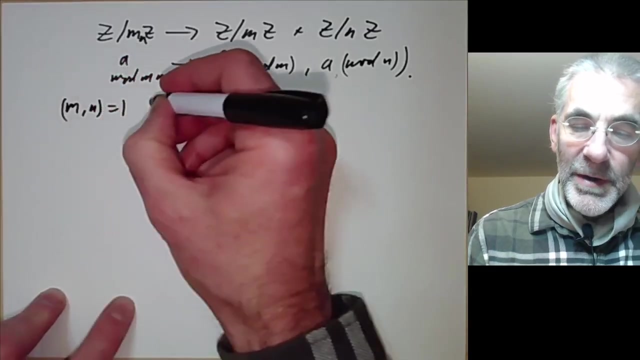 times z modulo n z. So this is a product of two sets and we're just mapping an integer, a modulo m n, and we're mapping it to a modulo m and a modulo n and we notice that if m n is equal to one, this is injective. 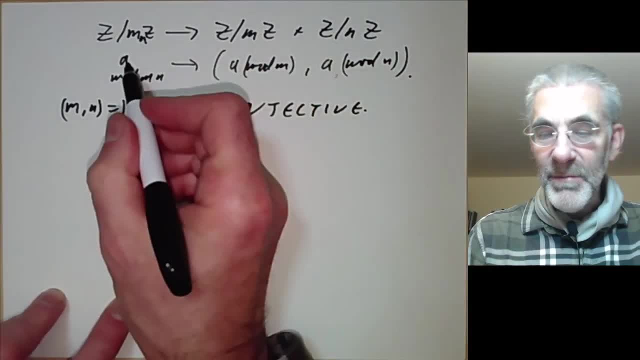 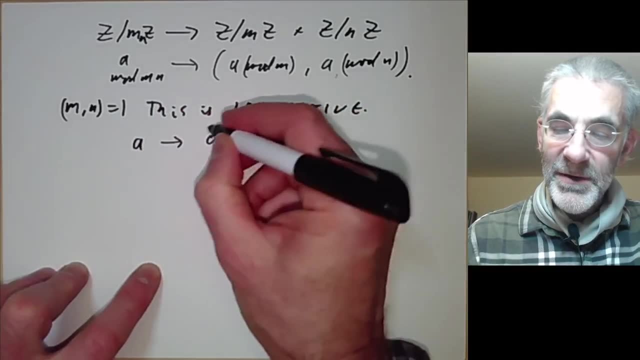 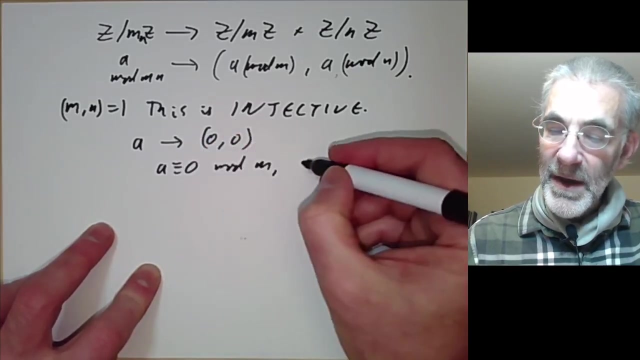 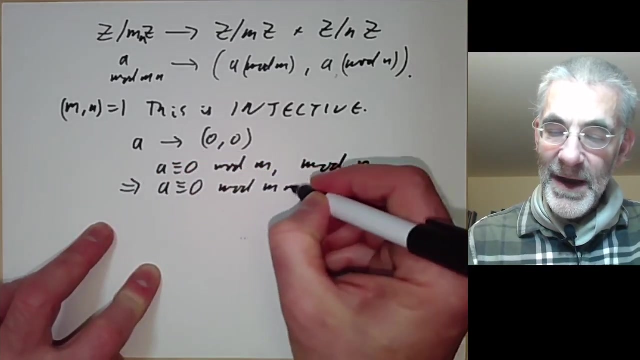 meaning there's at most one element here mapping to any element there. For example, suppose a maps to the element zero, Then this means that a is congruent to zero modulo m, and it's also congruent to zero modulo n. So a is congruent to zero modulo m n, and here we use the fact that m n are co-prime. 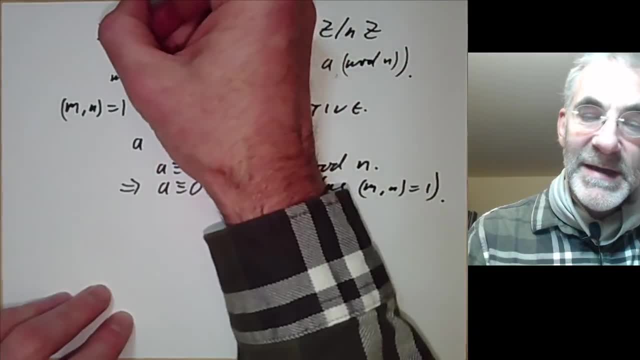 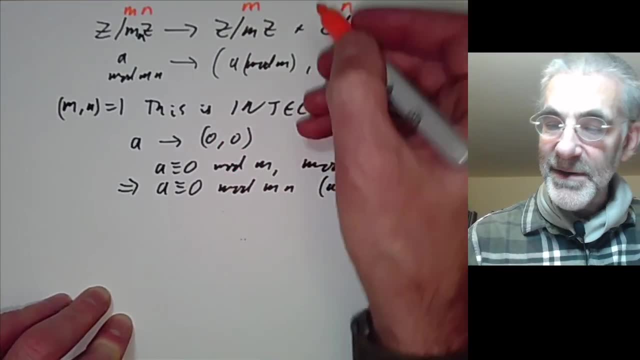 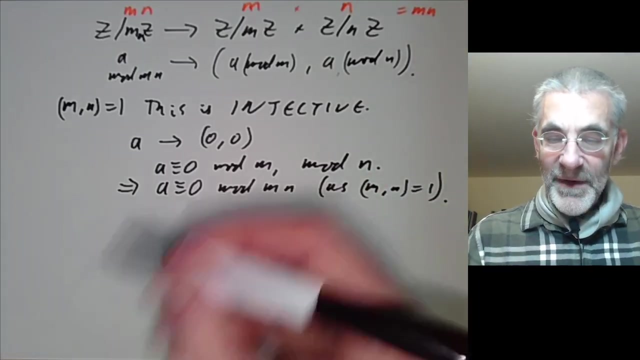 So it's injective. On the other hand, if you look at the size of these sets- this set of size m n and this set of size m- oops, and this set of size n, so this set here's size m times n, which is just m n of course. So we have an injective map. 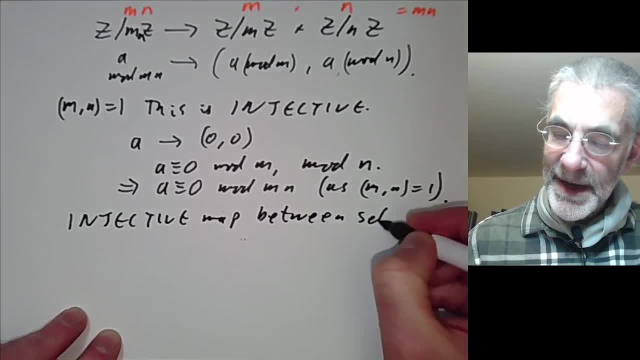 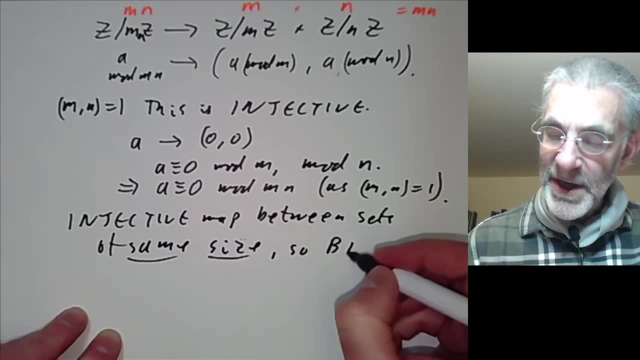 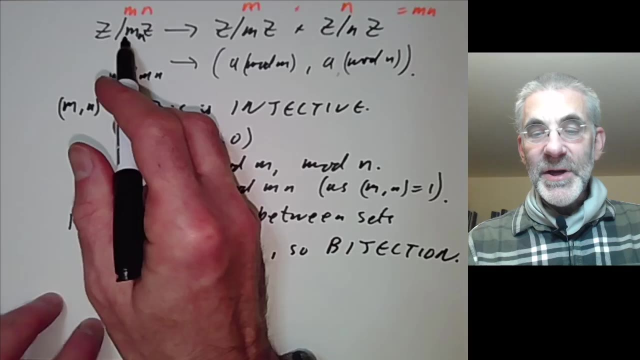 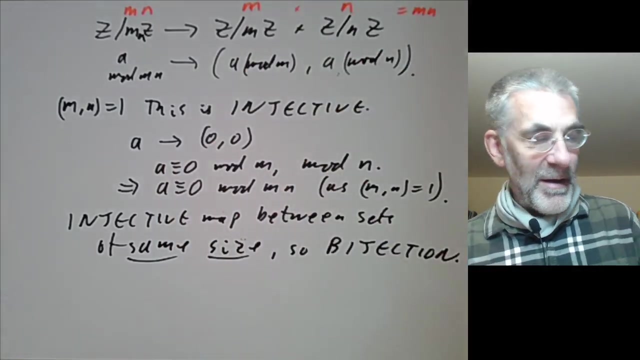 between sets of the same size. so it is a bijection. If you want to write this in terms of ring theory, we actually get an isomorphism of rings between this ring here and the product of these two rings here. I'm not emphasizing abstract algebra too much, but you could probably 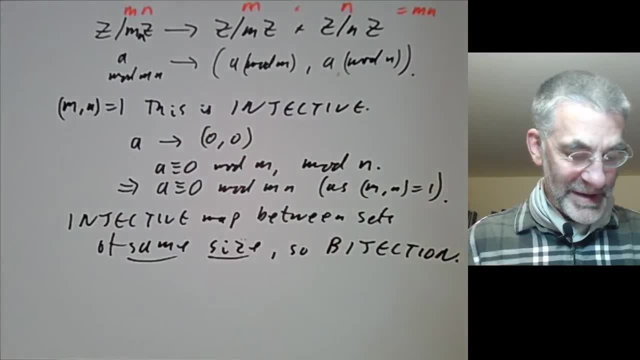 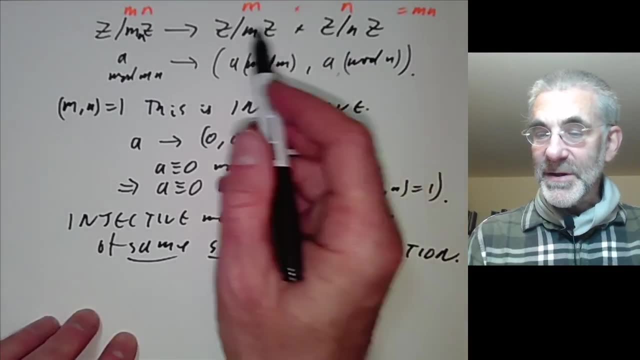 figure out what the product of two rings is and check that this is an isomorphism. Well, there's a bit of a problem with this, because suppose you've got an element z modulo m and an element of z modulo n, How do you find the? 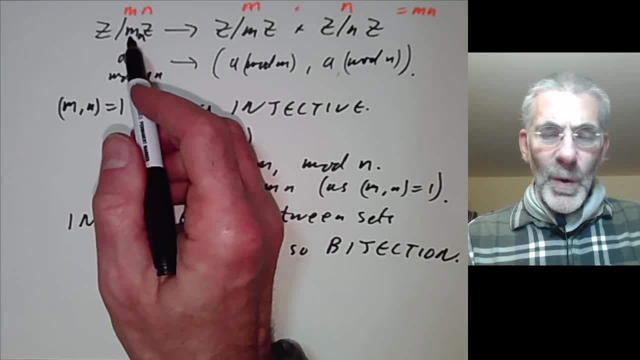 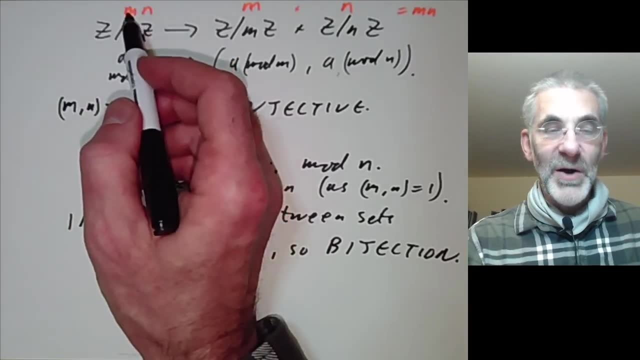 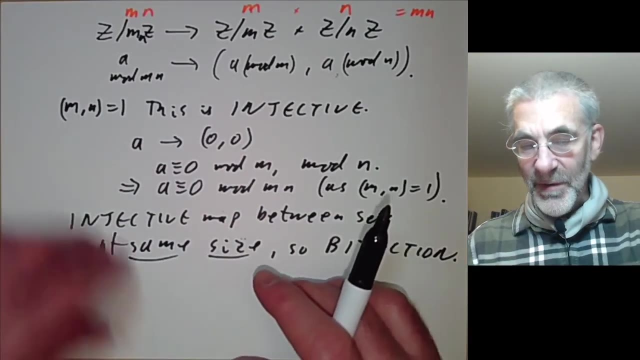 corresponding element of z modulo mn. Well, there's a stupid algorithm to do this. you could just check every element of this ring here until you find one that works. but if mn say, of a hundred digits, this is going to be ridiculously slow. Fortunately, there's a much faster algorithm, so what I'm going to do now is: 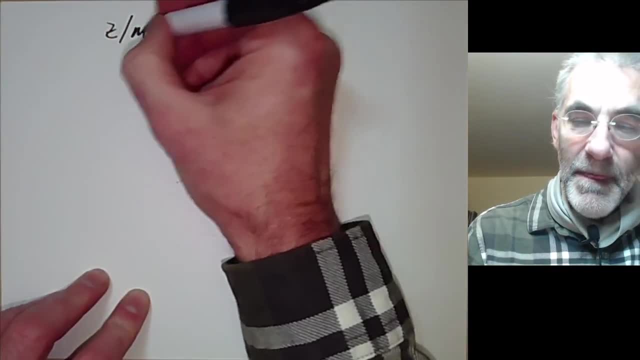 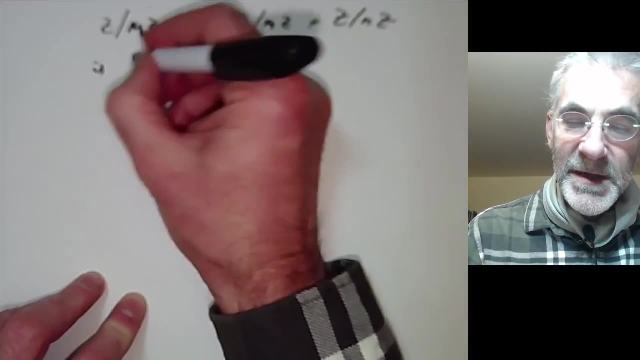 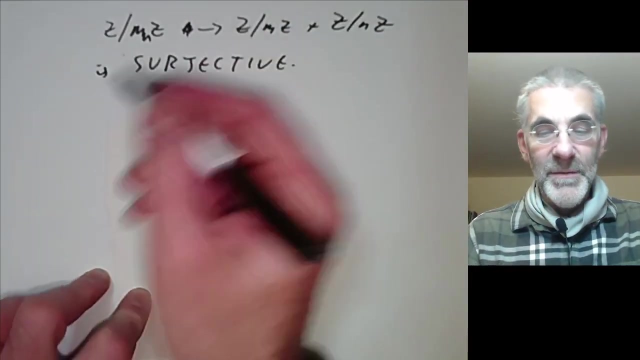 to show that z modulo mz- sorry, mz maps to z over mz times z modulo nz- is zero Surjective and I'm going to prove this in a way that actually gives you a fast algorithm. I mean, we've shown it's surjective by this rather abstract thing. 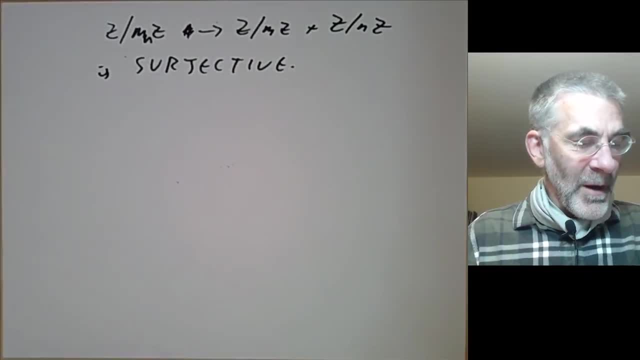 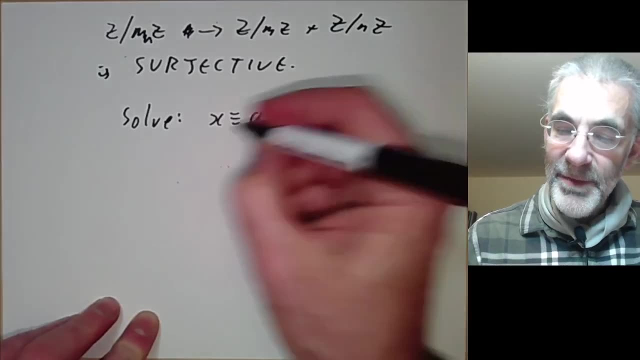 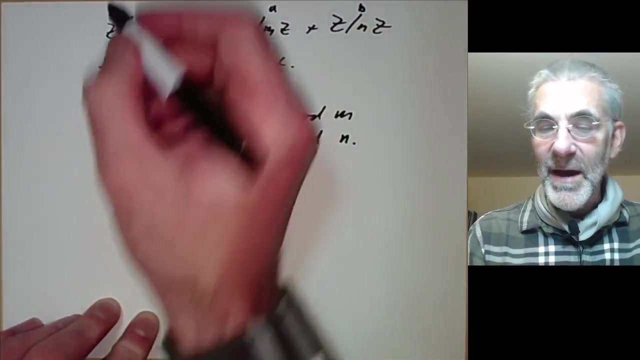 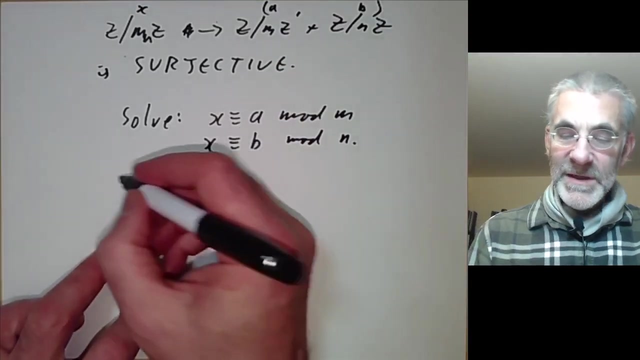 So what we want to do is to solve: x is congruent to a modulo m and x is congruent to b modulo n. So we might choose an element a here and an element b there, and we want to find an element x here which maps to a b. Well, let's think what this means. This means x is equal to a plus my. 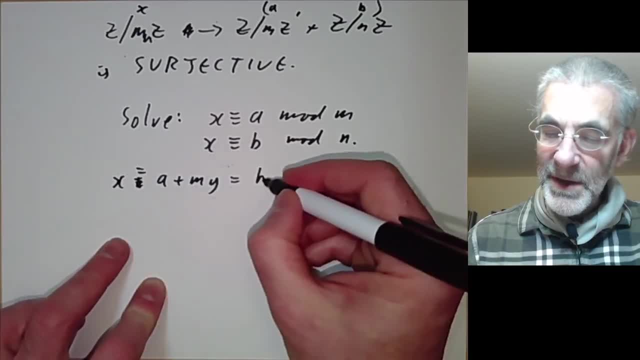 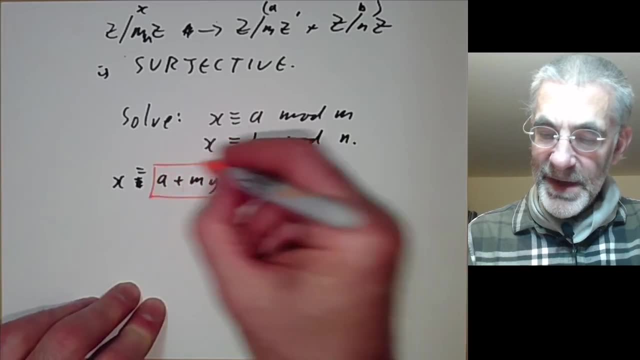 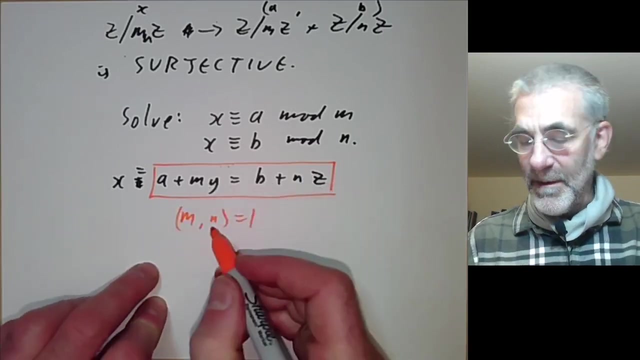 it's actually equal. and this also has to be equal to b plus n z. and now if you look at this bit here, we can see this is just a linear Diophantine equation and mn a 1, mn a co-prime, So we can solve a. 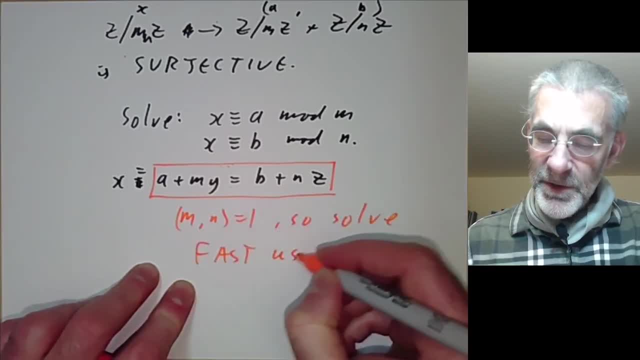 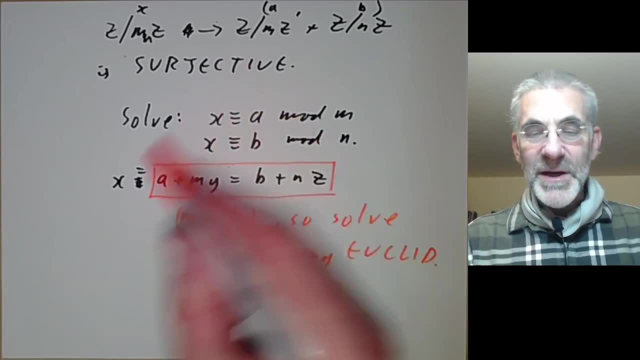 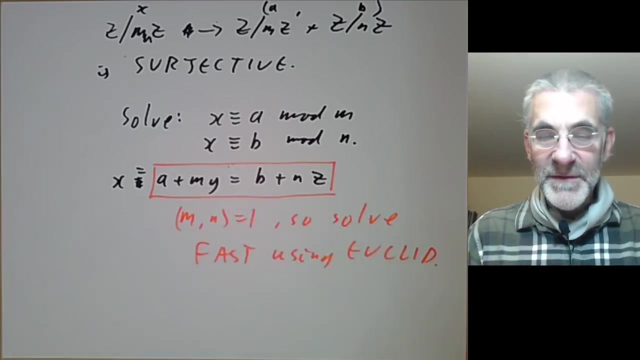 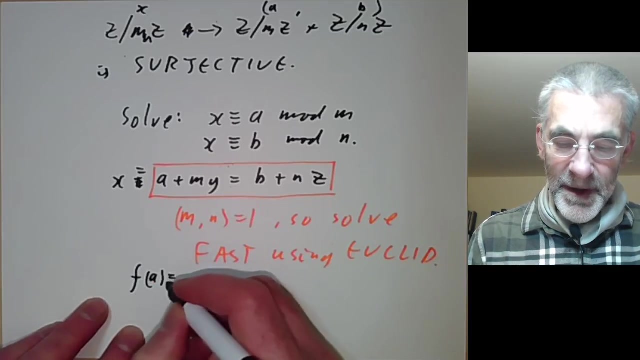 fast using Euclid's algorithm. So this proof and its surjective looks a bit more complicated than the previous proof we gave, because you've got to use Euclid's algorithm, but on the other hand it gives us a fast algorithm. And now this is useful because if we want to solve f of a is congruent to 0 mod mn, we 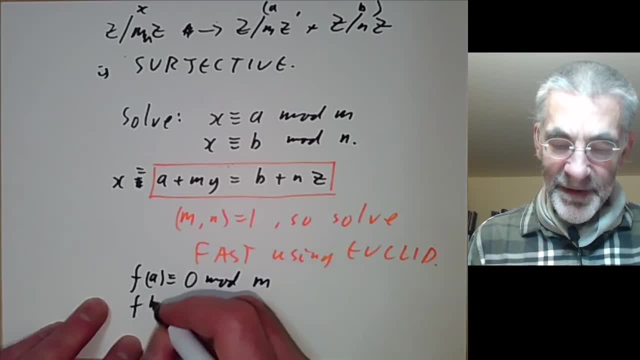 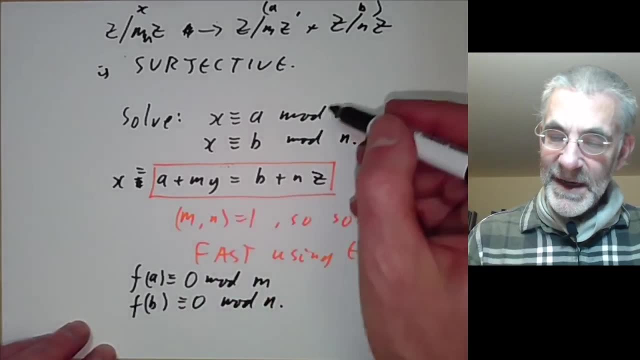 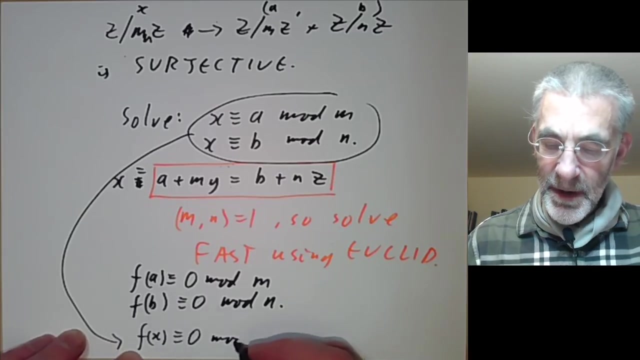 might solve: f of a is congruent to 0 mod m and f of b is congruent to 0 mod n, and then if we find an x satisfying these conditions here, then we will get f of x is congruent to 0 modulo mn. So by using this isomorphism we can reduce solving an equation modulo mn to 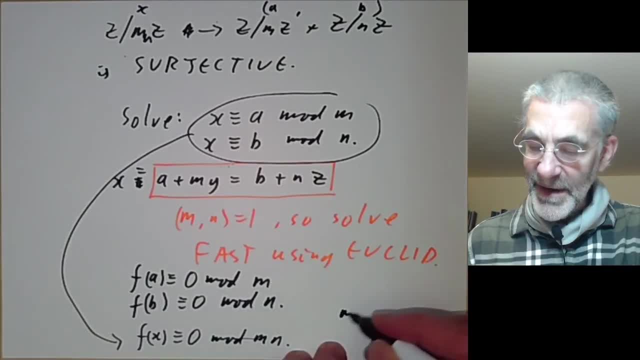 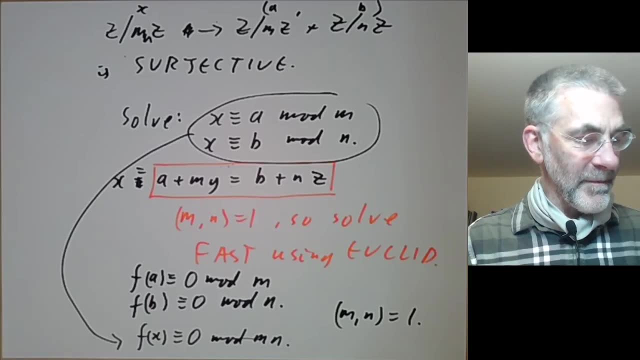 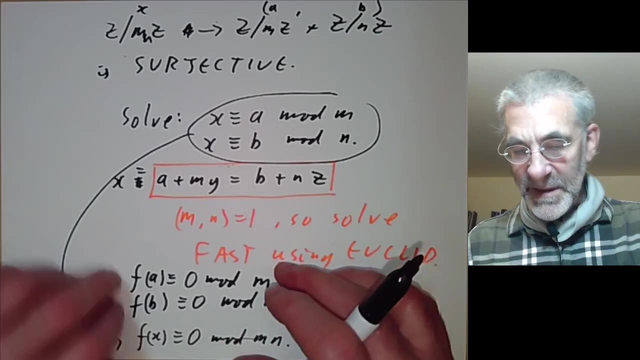 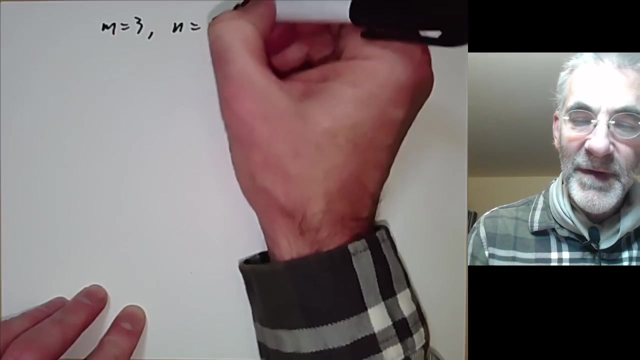 solving an equation: modulo m and modulo n. Again, as usual, m and n have to be co-prime. So let's write out an example of this explicitly, just to see what's going on, and then do a few examples. So let's take m equals 3 and n equals 5.. So we're looking at z modulo. 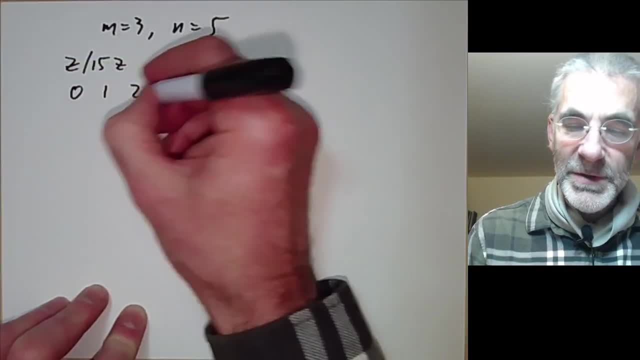 15 z, and let's just write out its elements: 0, 1,, 2,, 3,, 4,, 5,, 6,, 7,, 8,, 9,, 10,, 11,, 12,, 13,. 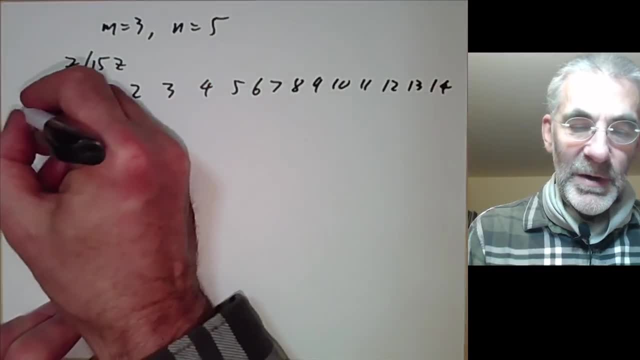 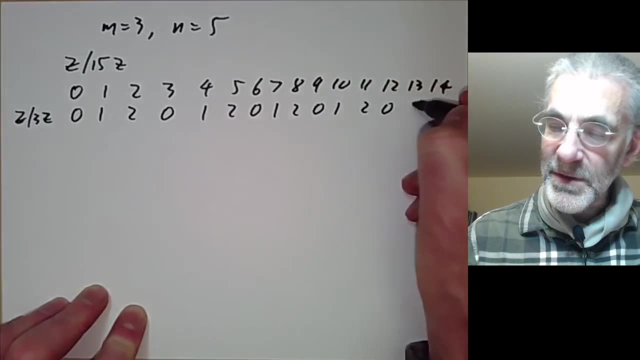 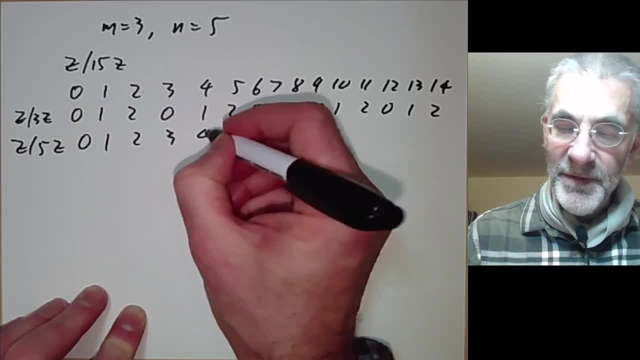 and z modulo 5z. so we get 0, 1,, 2,, 3,, 4, 0, 1,, 2,, 3, 4, 0, 1,, 2,, 3,, 4.. So you see that. 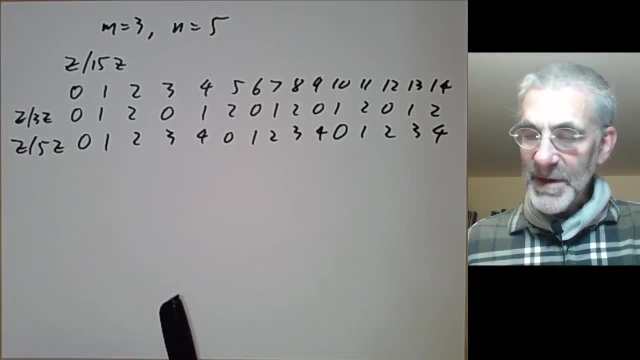 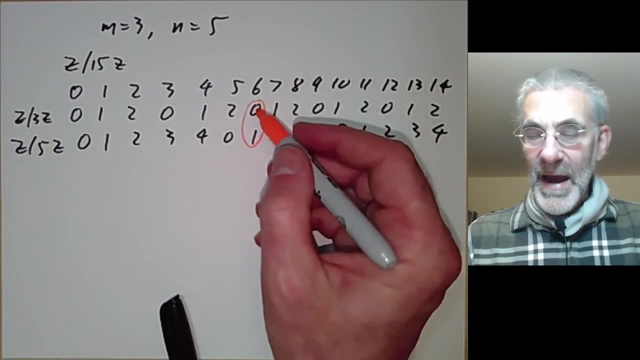 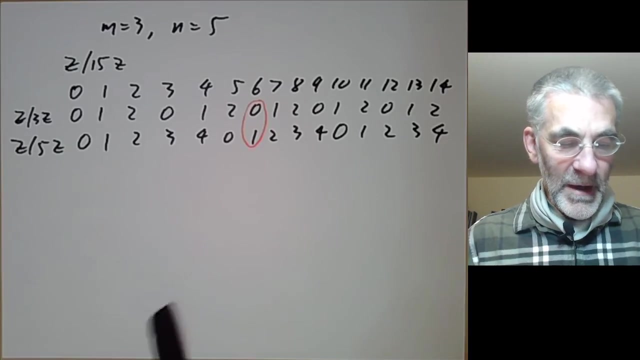 for every pair of elements here. so if we take the element 0 here and 1 here, there's a unique column containing that pair. So x equals 0 mod 3 and 1 mod 5.. We look up the solution. it would be x is 6 mod 15.. 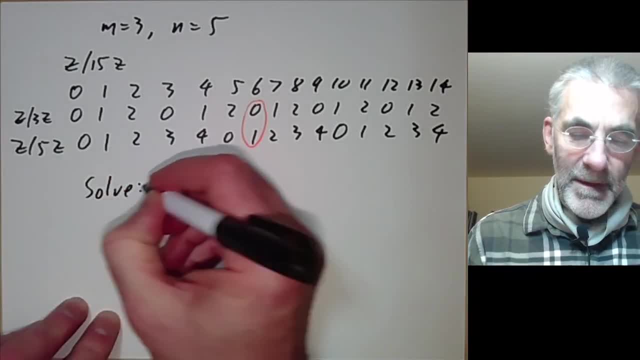 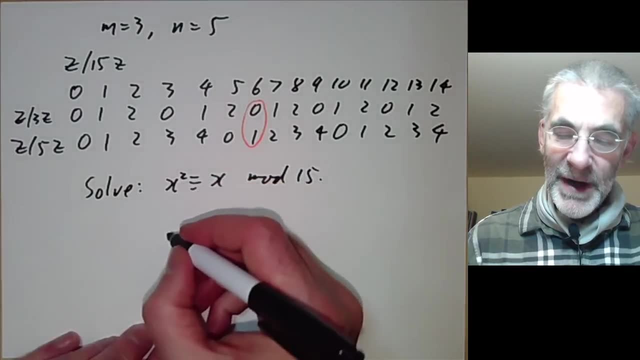 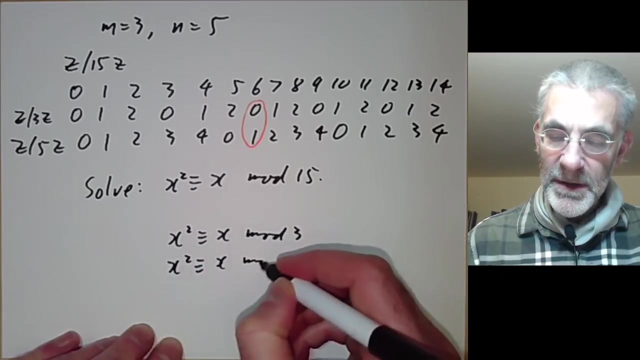 So let's solve: say, x squared is congruent to x mod 15.. So what we do is we break this into two problems. We solve: x squared is congruent to x mod 3 and x squared is congruent to x mod 5.. 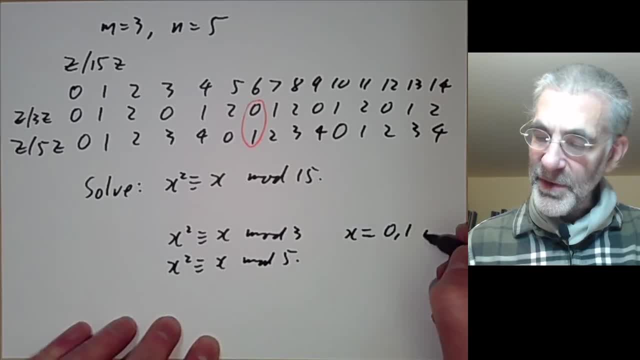 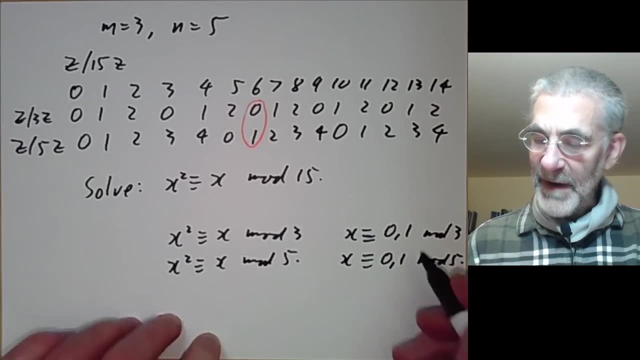 And then we see that x has to be congruent to 0, 1 mod 3 and x is congruent to 0, 1 mod 5.. However, the 0, 1 here doesn't have to be the same as the 0, 1 there. All this says: 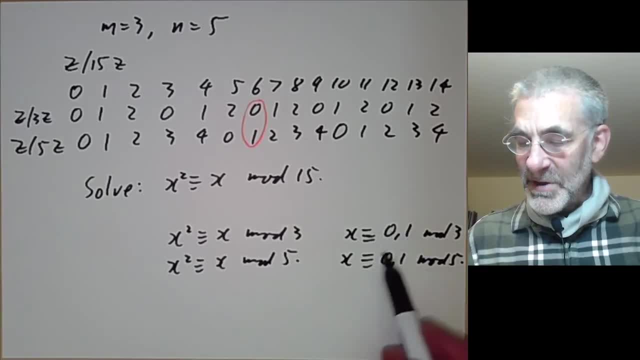 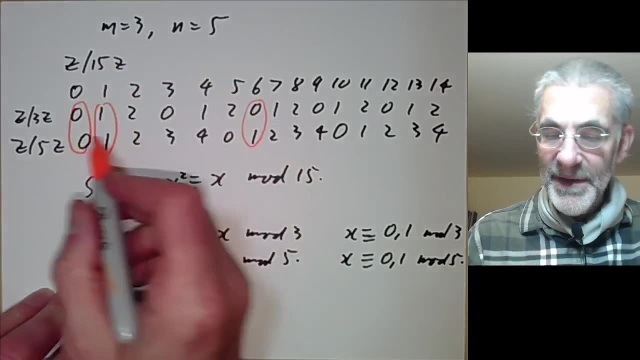 is that x must be 0, 1 mod 3 and it must also be 0, 1 mod 5.. And if we look in this column, we see that there are four solutions to that. There are two obvious solutions, but there. 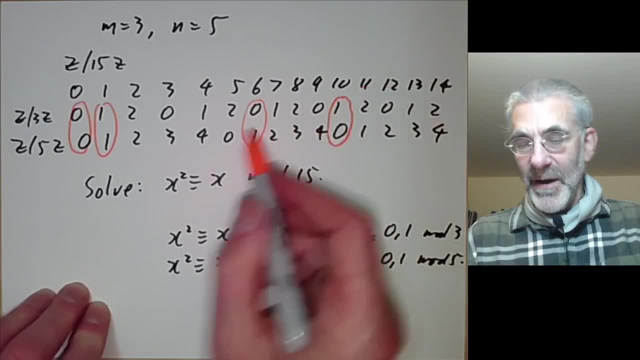 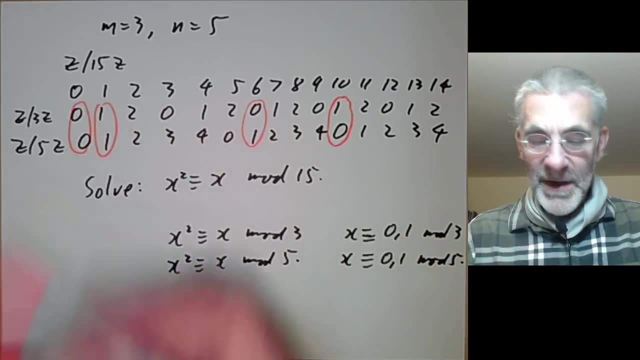 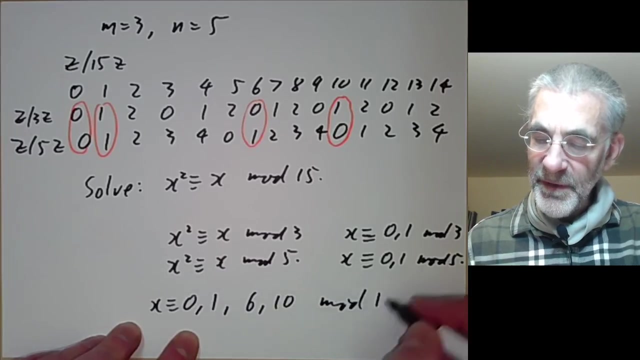 are two slightly less obvious solutions. So there we find the columns where we get 0 or 1 in this row and 0 or 1 in this row, And so we see that gives us x is congruent to 0,, 1,, 6 or 10 mod 15.. 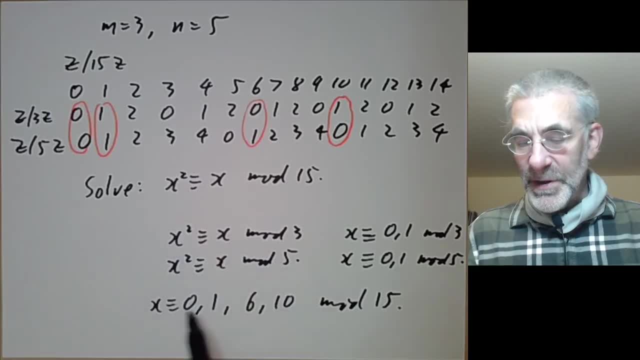 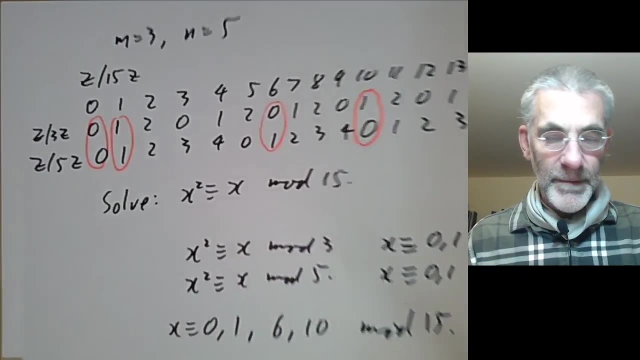 Notice, by the way, that here we've got a quadratic equation which has four roots. So if you're used to equations of degree 2 having only two roots, that actually fails if you're working modulo 15.. We've discussed that in more detail a bit later. 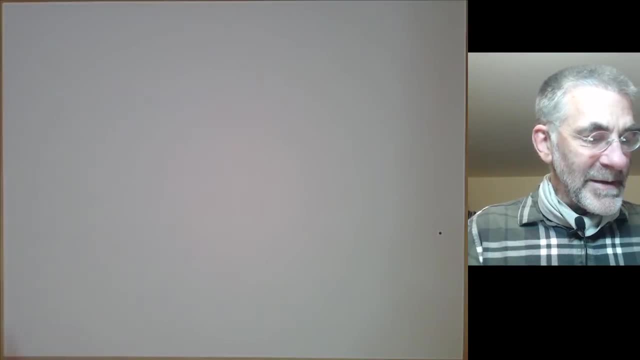 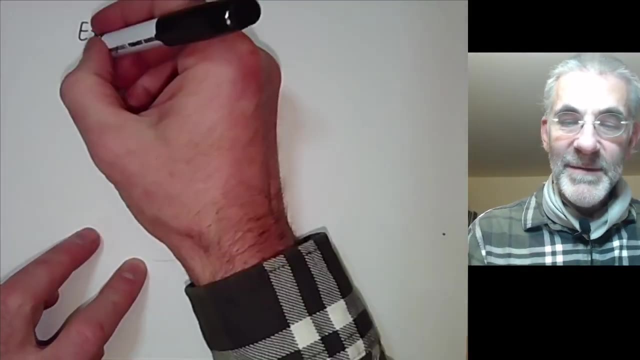 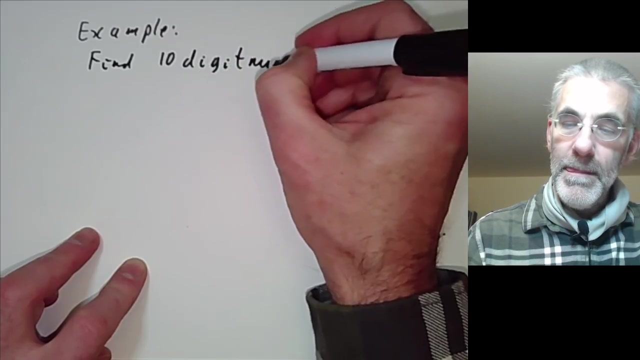 So another similar example. Let's have the following recreational mathematics problem: Find a 10 digit number, number x, so that x mod 3 is congruent to x mod 5.. Then we find that x is congruent to x mod 5.. And 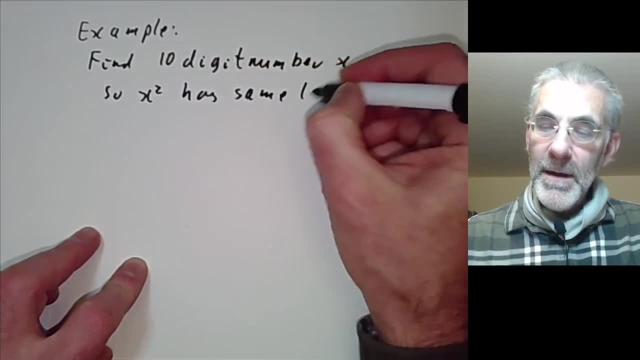 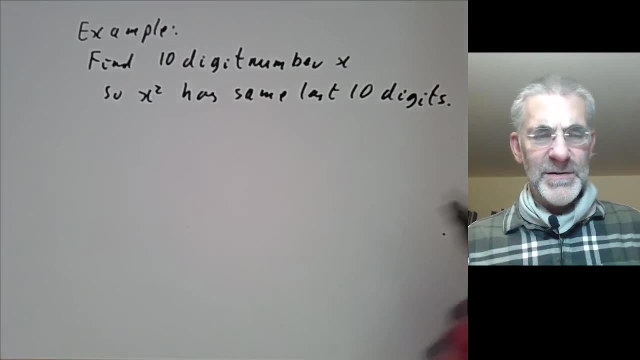 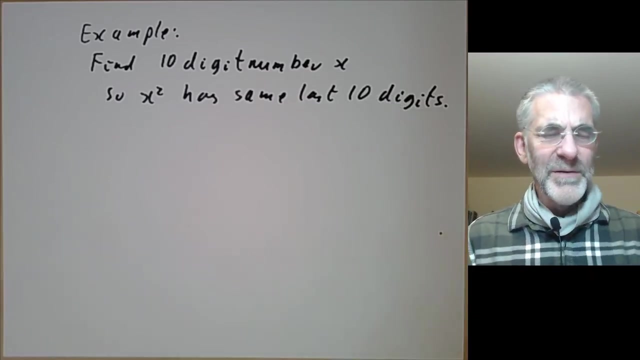 squared has the same last 10 digits. here we're working to base 10 and you know this problem depends on working in base 10 and most problems that depend on working base 10 are kind of a bit silly, you know. you get these problems like: 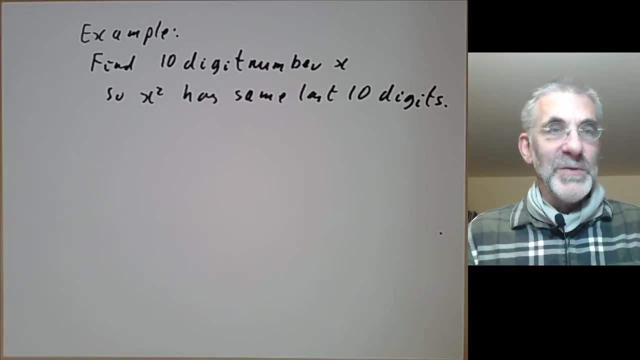 find a number that's the sum of the cubes of its digits or something. and most of these problems are of no mathematical interest whatsoever, because as soon as you change base, the problem becomes completely different. but that this one. it actually leads to some slightly interesting mathematics. so 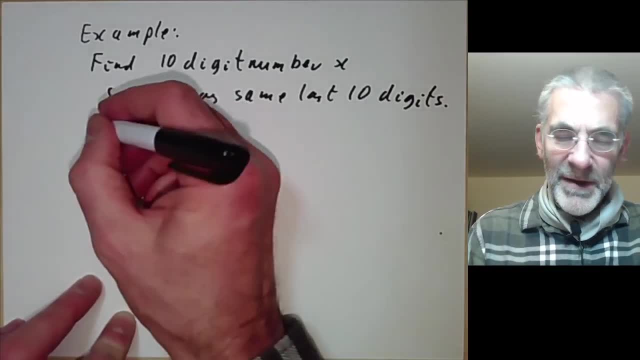 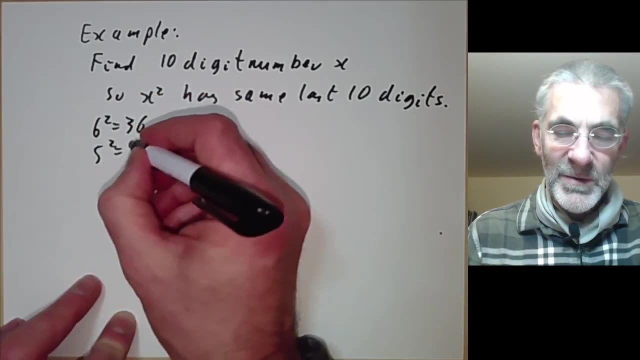 instead of making the last 10 digits the same, let's just try and make the last digit the same. well, here we can get: 6 squared equals 36, the last digits the same: 5 squared equals 25. well, we can cheat, of course. we can take X to be 0, or 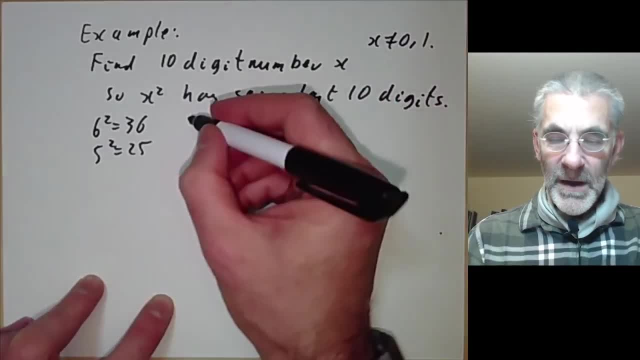 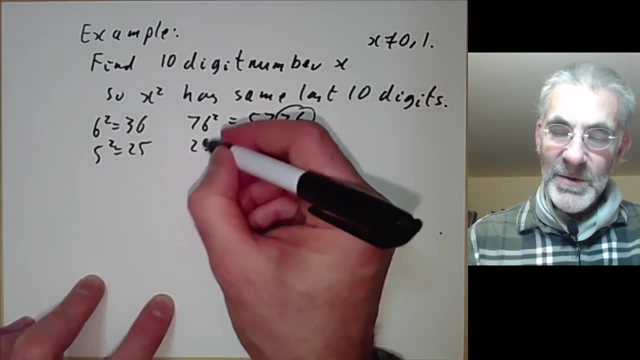 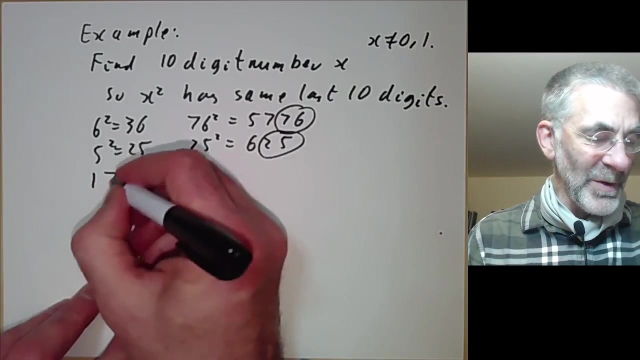 1, so let's just say X is not equal to 0 or 1. and then 76 squared is 5, 7, 7, 6, last two digits the same. 25 squared is 6, 25, last two digits the same. and we can go on like this and we find, for example, at one, seven: 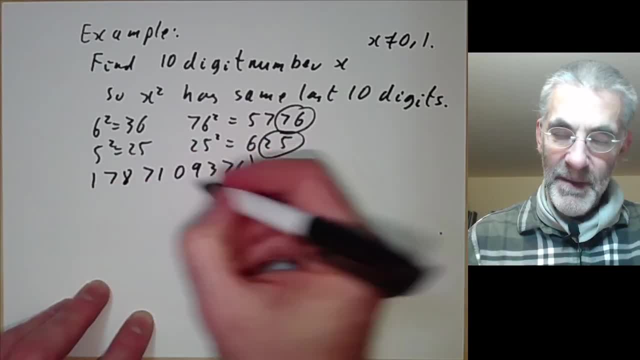 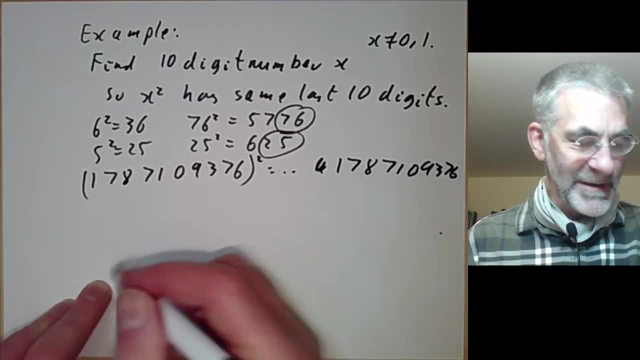 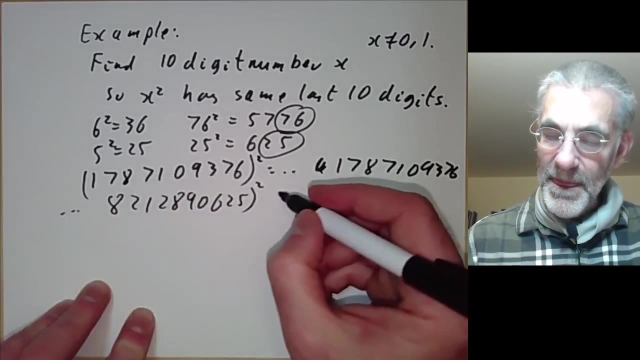 eight, seven, one, oh, nine, three, seven, six. squared is something or other: one, seven, eight, seven, one, oh, nine, three, seven, six. and similarly, if we take eight, two, one, two, eight, nine, oh, six, two, five squared is: This has the same last digits that I'm not going to bother writing out. So the problem is: 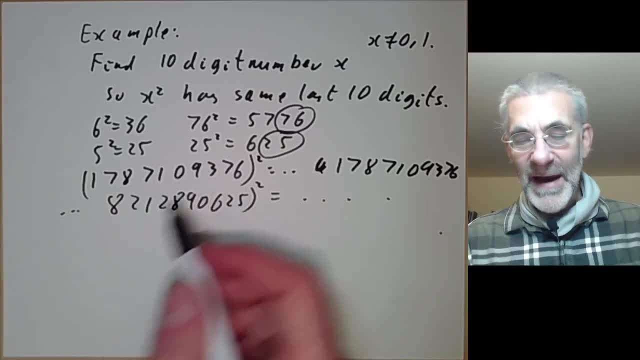 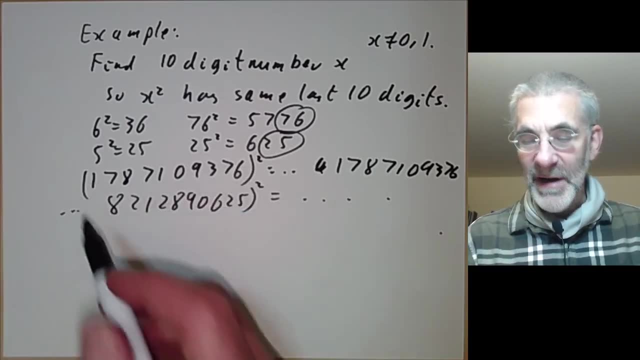 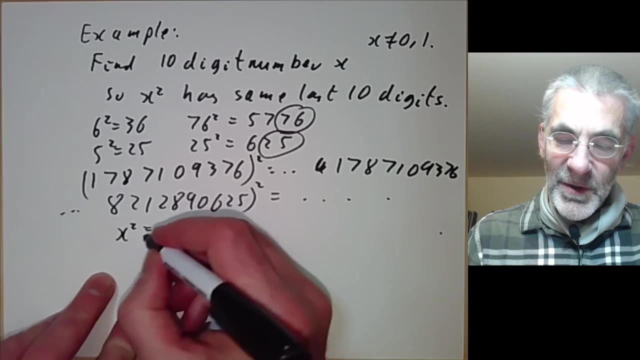 how do we find these numbers? Obviously, trial and error is going to be a well. These days, computers can do billions of operations a second, So trial and error is probably the fastest way to do it. but never mind anyway, If we do, x squared is congruent to x. 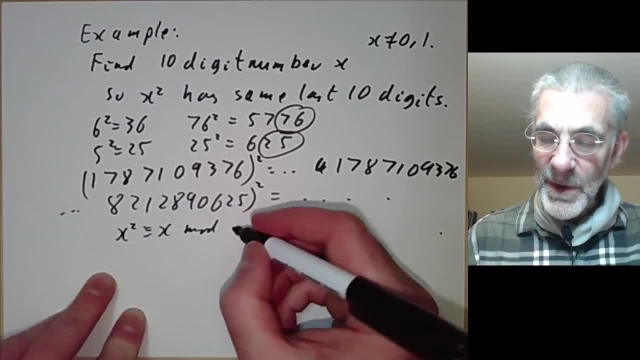 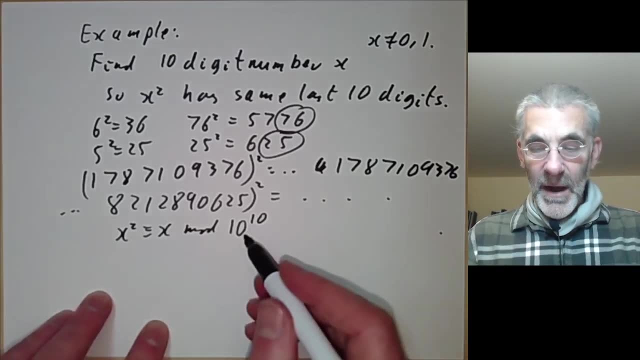 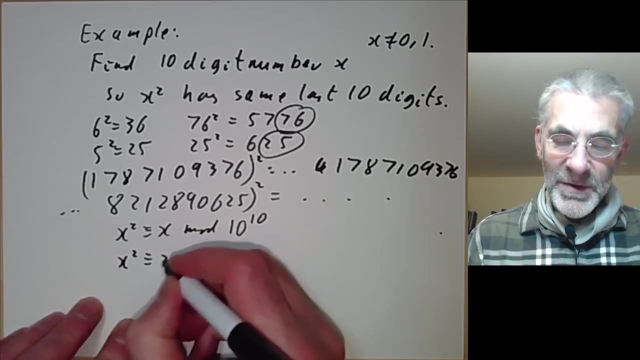 What we want to do is to solve x squared is congruent to x modulo 10 to the 10. that just says x squared and x Have the same last 10 digits. Now we notice the Chinese remainder theorem applies to this. This is the same as solving x squared is congruent to x. 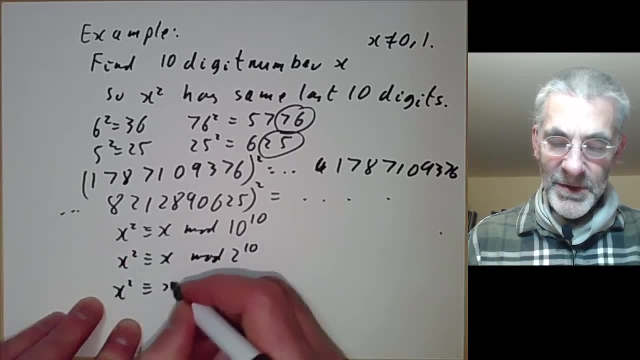 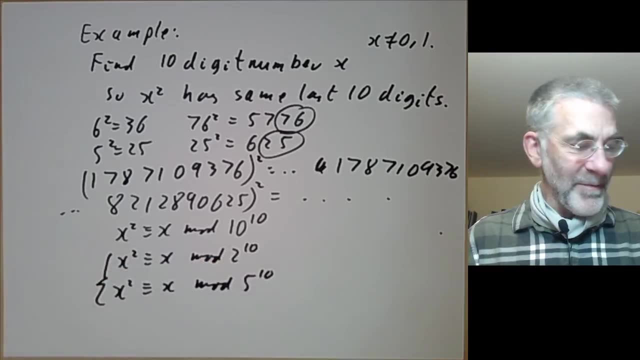 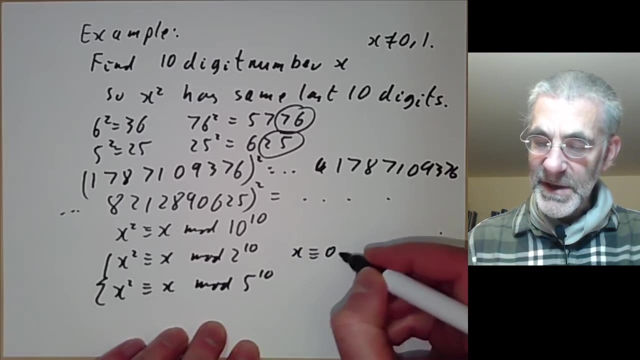 modulo 2 to the 10, x squared is congruent to x modulo 5 to the 10. So we've reduced it to two Equations, each modulo of prime power and each of these we can think of some solution. So x is congruent to 0 or 1. 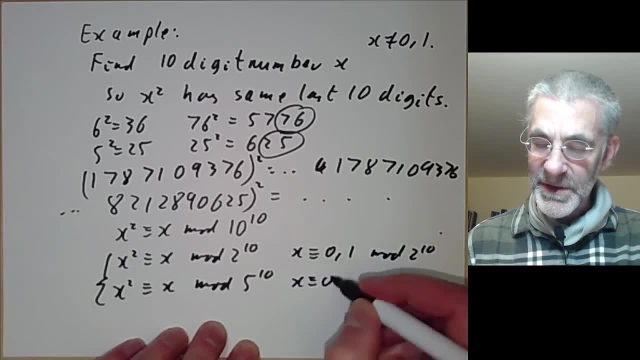 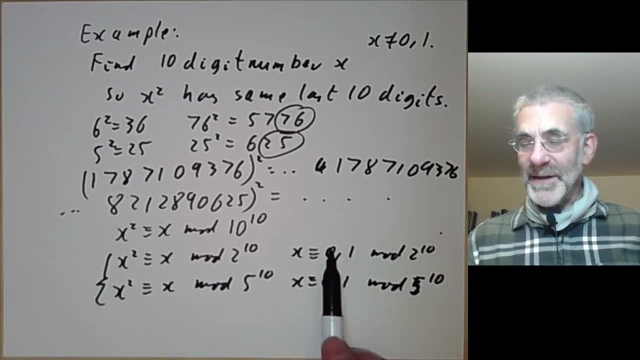 Modulo 2 to the 10, and this has solutions: x is congruent to 0 or 1. modulo 3, 5 to the 10, And now we could take x 0 in both of these, and that would give us the uninteresting solution 0 and we could take 1. 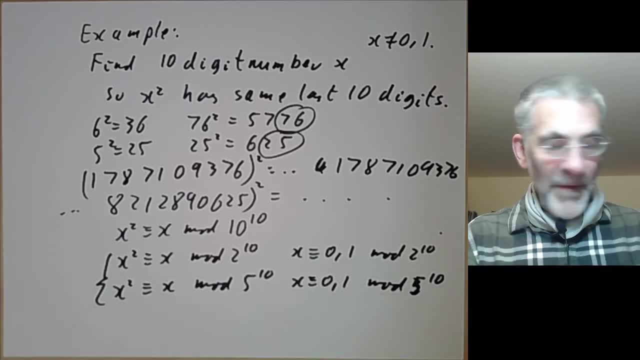 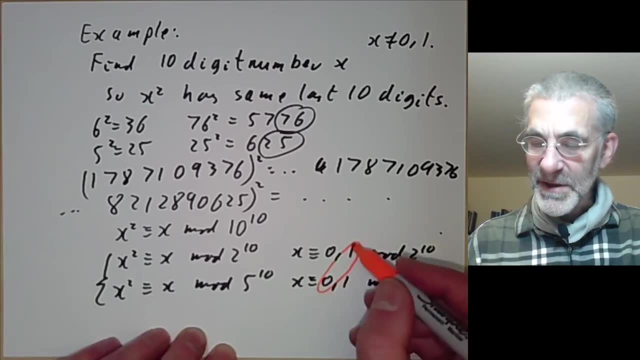 And that would give us the uninteresting solution 1.. However, we can sort of take cross terms, So I can take x congruent to 0 mod 5 to the 10 and 1 mod 2 to the 10, And that gives us this solution which we can work out using. 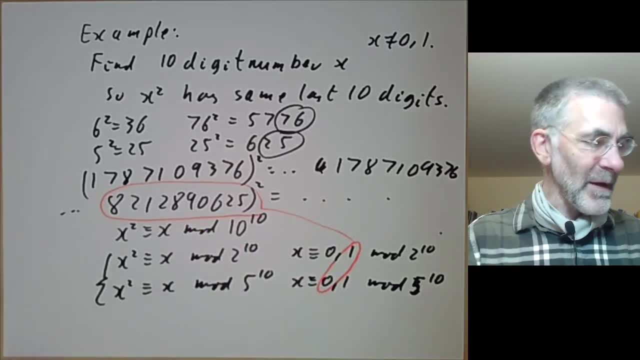 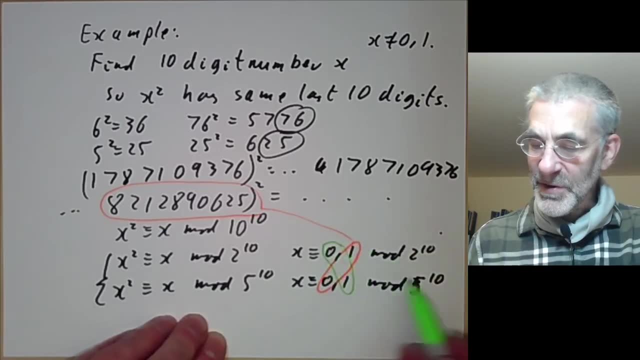 Euclid's algorithm, if we want, And actually there's another way that I'll mention in a moment. Alternatively, we can take these cross terms: We take x common to 0 mod 2 to the 10 and 1 mod 5 to the 10, and that gives us this solution here. 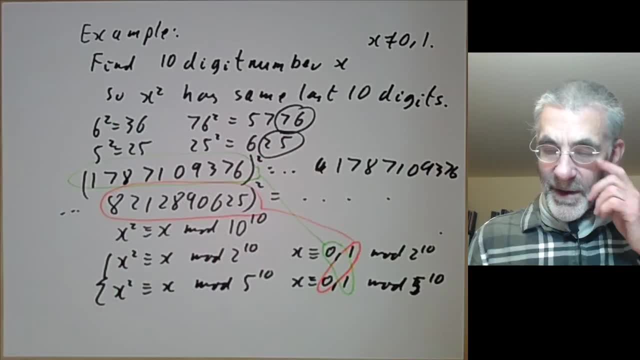 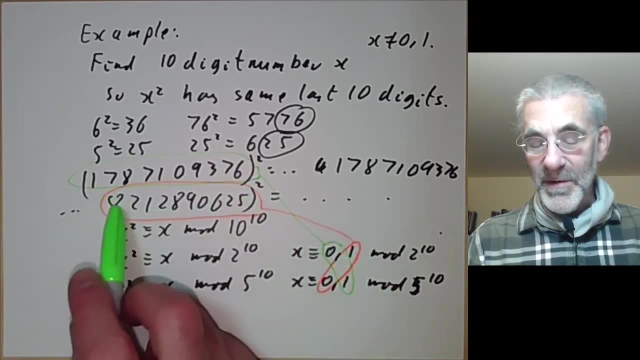 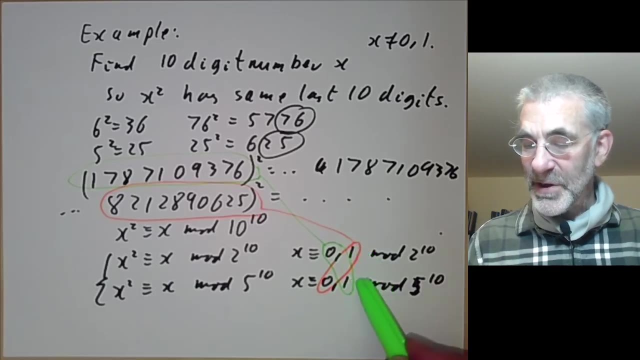 Incidentally, if you add these up, you'll suddenly notice that you get something Who, which ends in a lot of zeros followed by 1, and that follows because if you add these up, It would be something that's 1 modulo 10 to the 10. 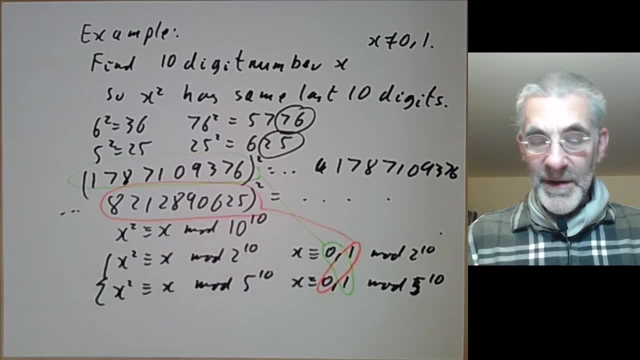 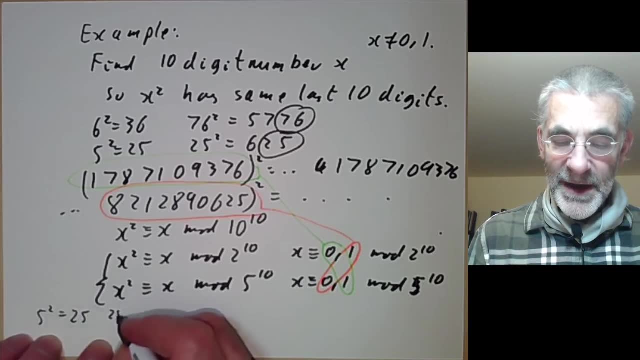 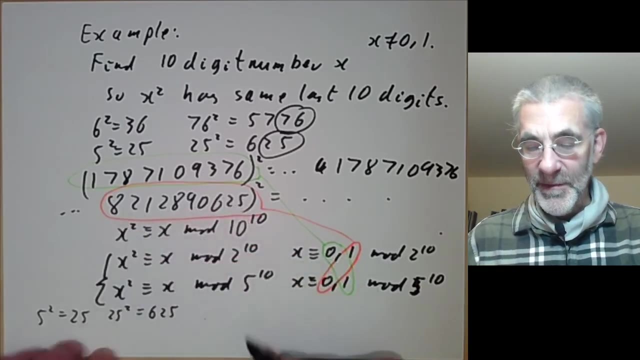 Anyway, I mentioned there was actually a different way of finding these solutions. what you can do is you can take five and then you can square it, and then you can square it again, and each time you square five you get an extra digit of this solution. so we can just carry on like this and I'm going to 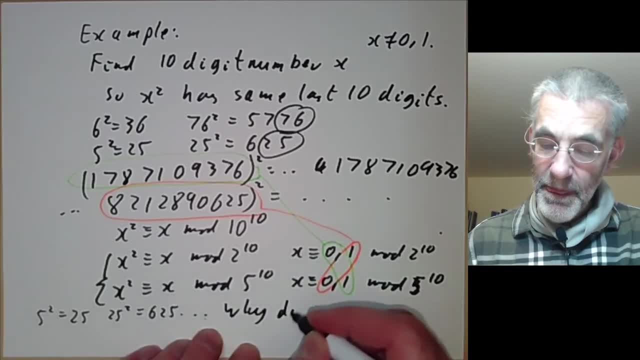 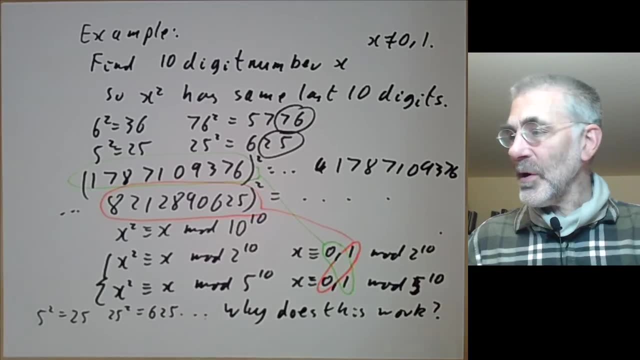 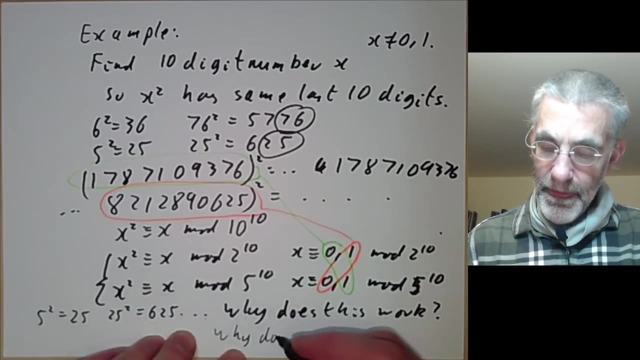 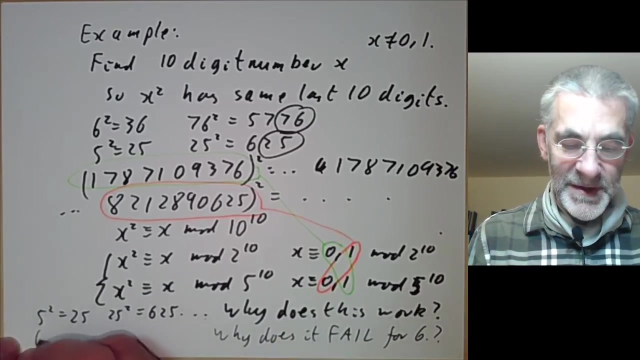 leave it as a little exercise. why does this work? and if you figure out why that works, I'll now have another exercise. why does it fail? for if you start at 6 rather than 5, so if we start at 6, we start with 6, squared is 36 and that's. 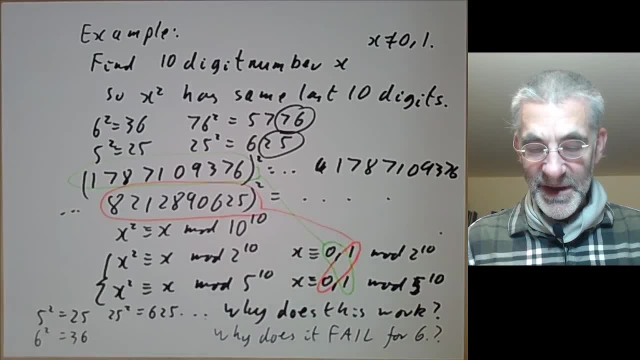 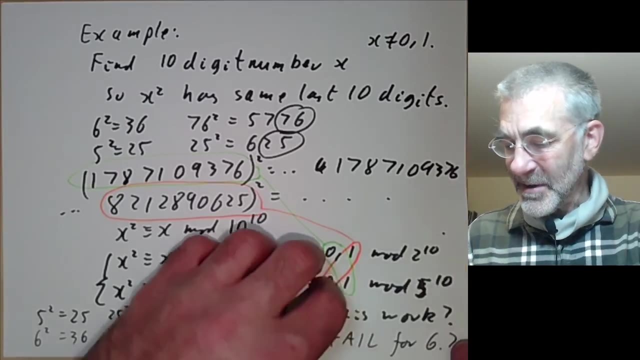 not giving us something ending in 76 so you can try and figure out what the difference between 5 and 6 is, which makes this thing work for just one of them, so Cut. Next example is going to be a historical example, which is sort of why this thing. 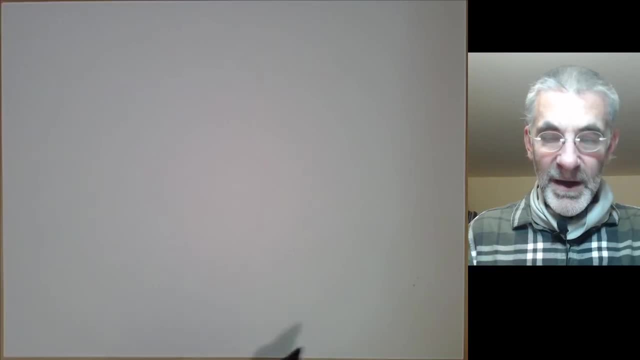 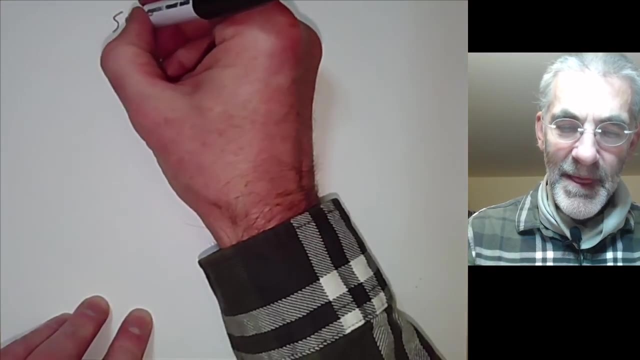 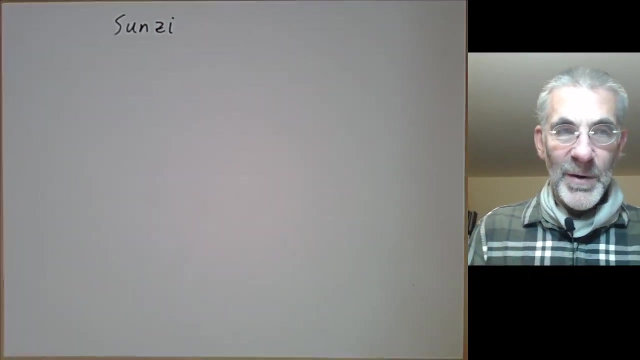 is called the Chinese remainder theorem. so this is a problem due to a Chinese mathematician and I can't write Chinese and his name is sometimes spelt as this: I'm not going to dare pronounce it because I've no idea what the tones are and if I, if I try and pronounce it, I'll probably say a bad word in Chinese and 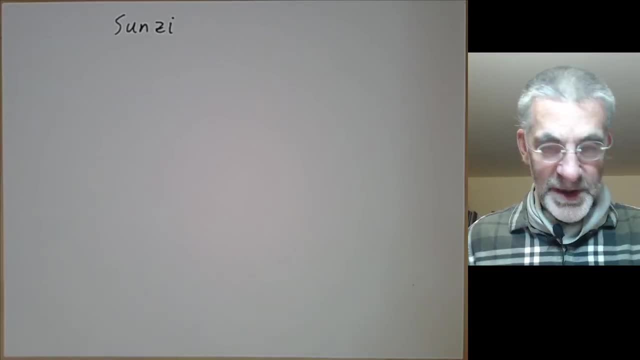 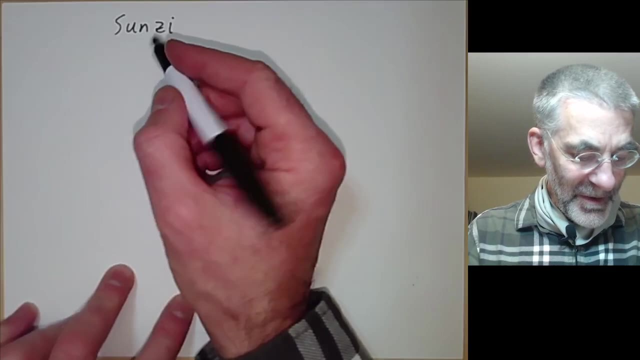 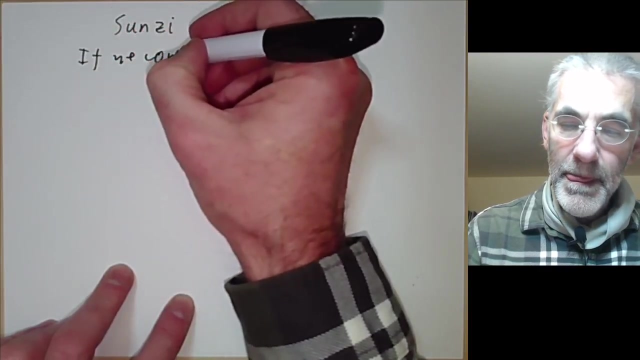 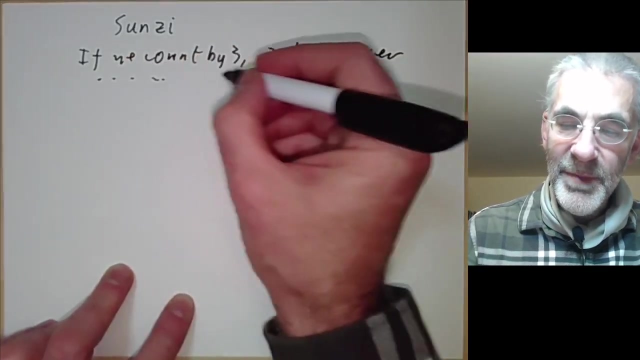 everybody who knows Chinese will start laughing at me. so anyway, he works. I mean about the third century and he had the following problems. suppose we have a number of things: if we count by three, there are two left over, and if we count by five, there are three left over. and if 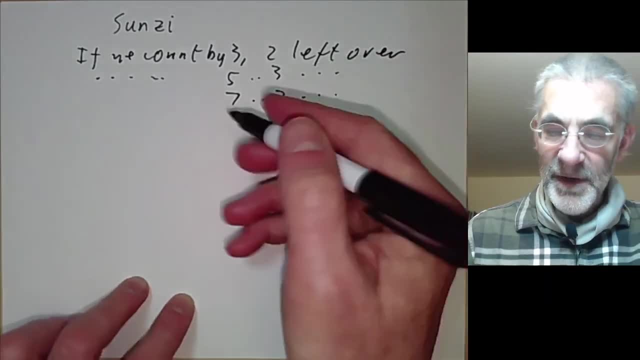 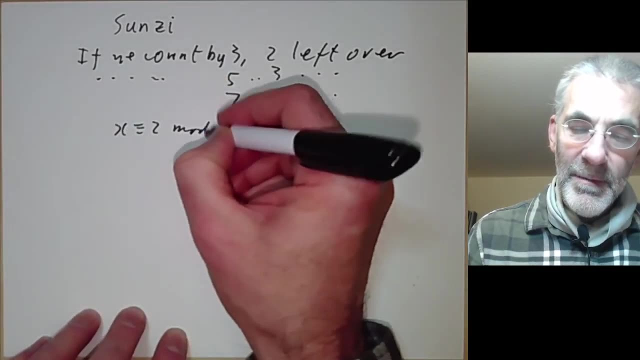 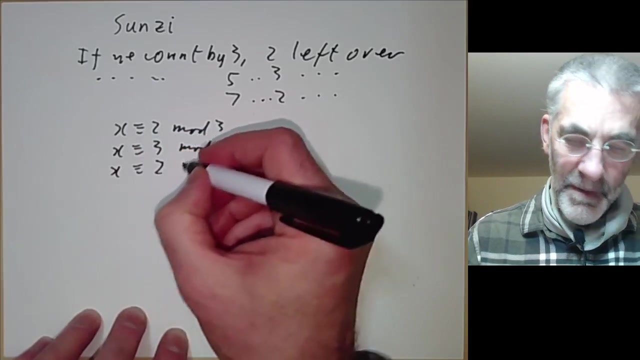 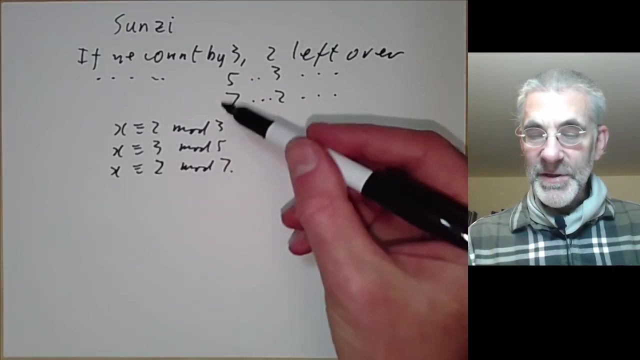 we count by seven, there are two left over, and the problem is to find out how many things there are. well, obviously, this is just solving the equation: X is congruent to two modulo three, X is congruent to three modulo five, and X is congruent to modulo seven. so here, instead of having two equations with 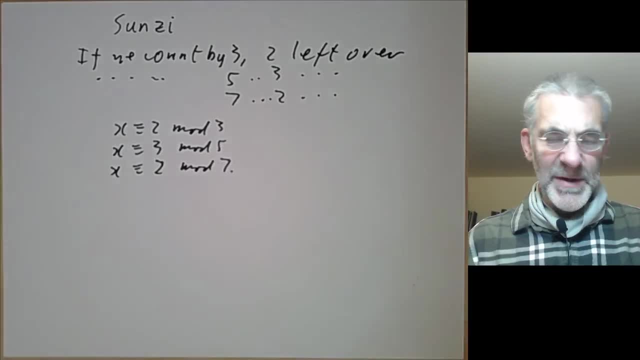 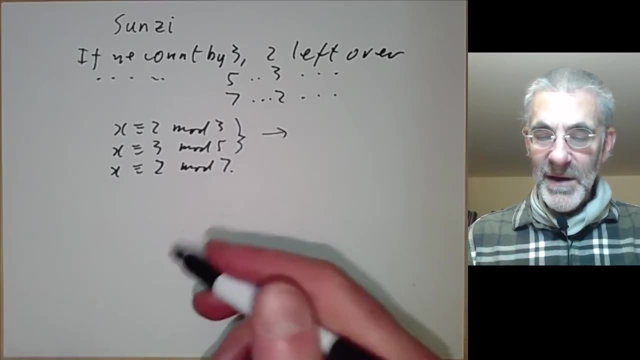 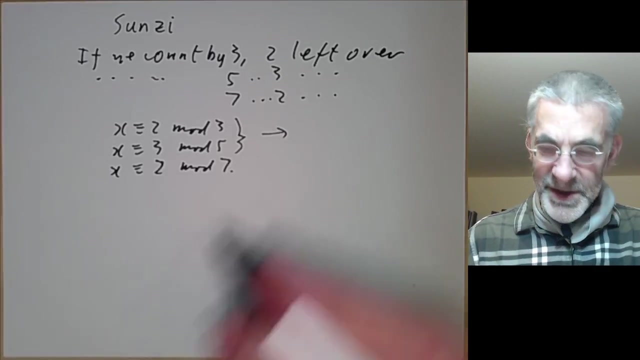 co prime numbers. we have three equations. so what do we do? well, well, obviously we first solve these two equations. here, three and five are co prime, and if we solve these you could use Euclid's algorithm. but frankly, for numbers as small as this, it's quickest just to just to guess, and you find this implies that X is congruent to 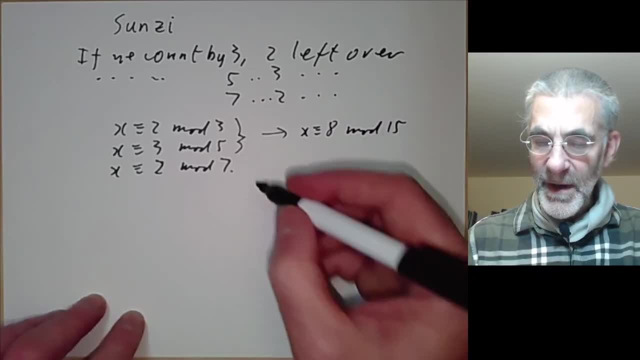 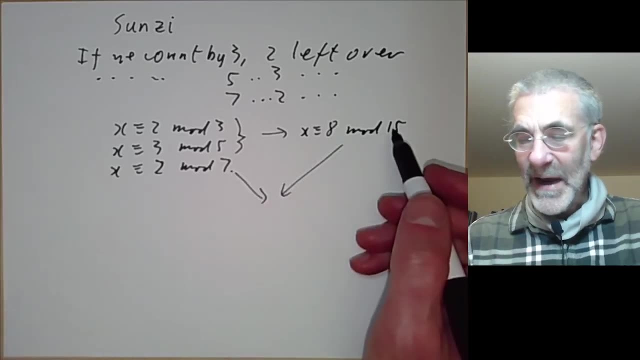 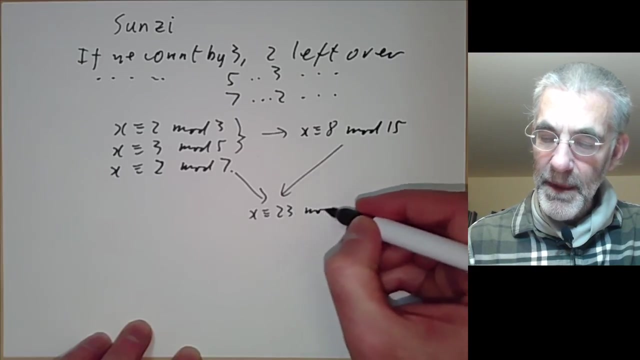 8 modulo 15.. so next we solve X congruent to 8 modulo 15, and X is congruent to 2 modulo 7. and again we could use Euclid's algorithm, but you can just cheat and guess and you find X is now congruent 23 modulo 7 times 15, which is 105. so the general solution of 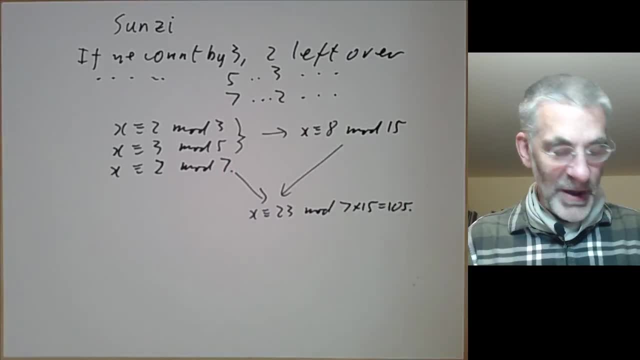 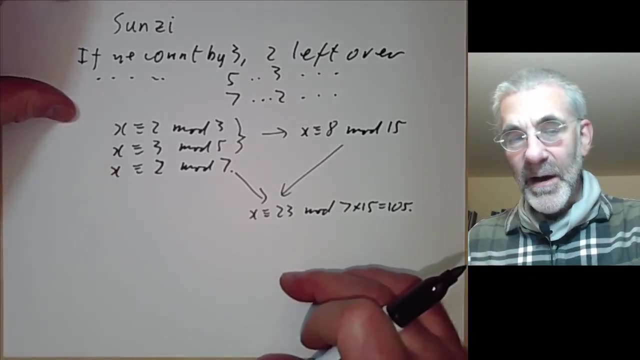 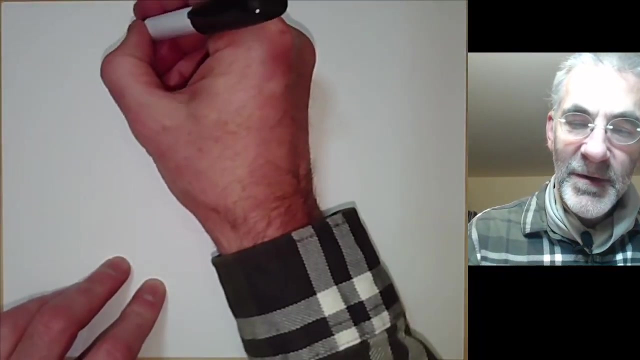 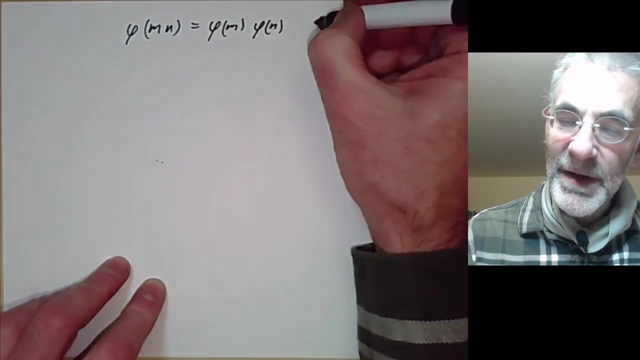 this is the number of things- is 23 modulo 105. now, earlier I showed that there was this identity for Euler's phi function, which says that phi of m? n is equal to 5m times five N, whenever m and n co-prime, and you can sort. 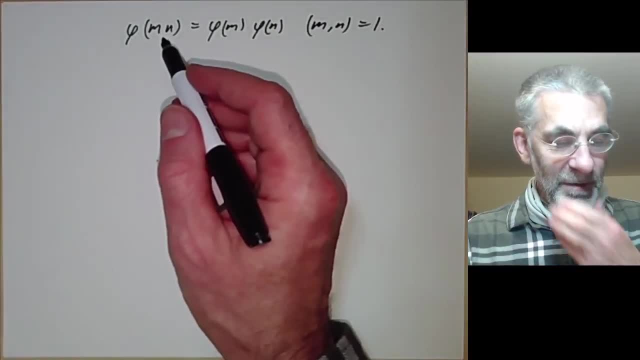 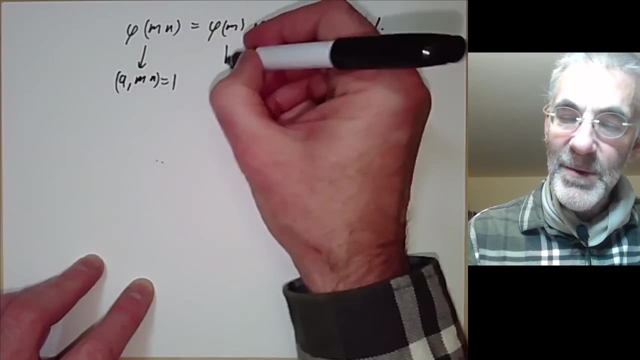 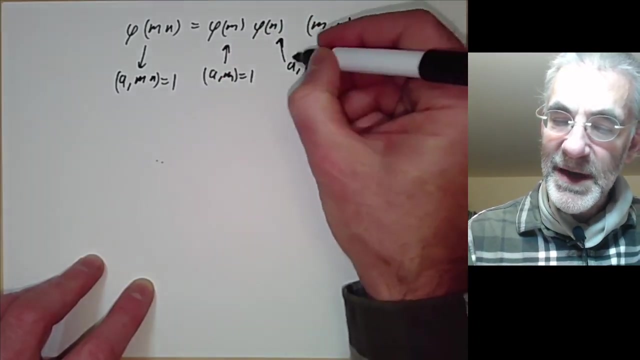 of prove this using the Chinese remainder theorem as follows: so so. so here we just count the numbers with a m, n equals 1, and here we kind of the number of things with a m, a co prime to M, and here we want a co-prime to N. and if we 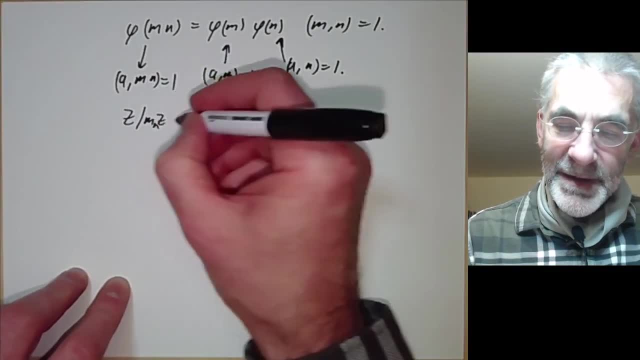 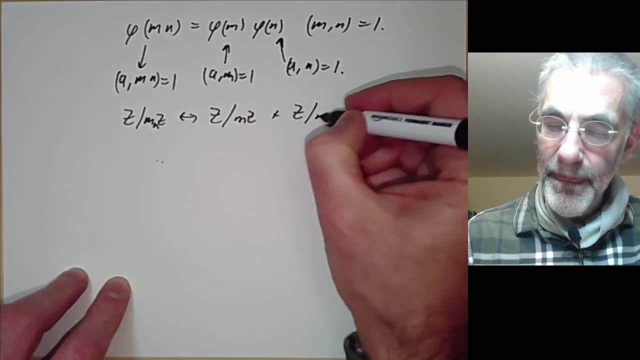 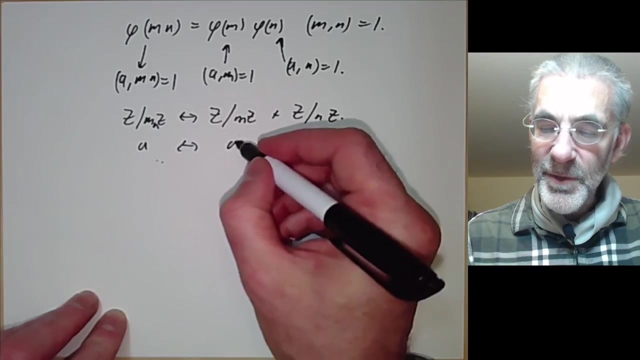 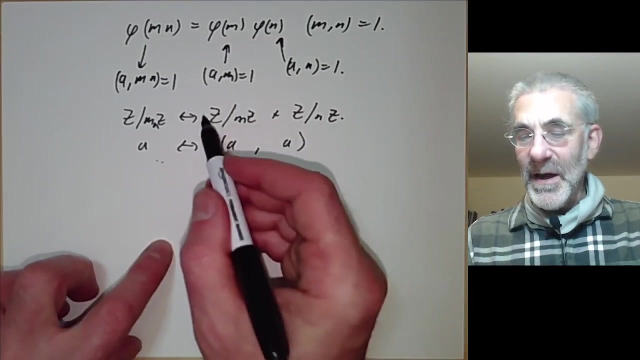 If we think of mapping Z modulo MNZ, we think of the isomorphism between these, we see that A is coprime to MN if, and only if, it's coprime to M and also coprime to N. So what we have to do is we can get any A coprime to MN by choosing something coprime. 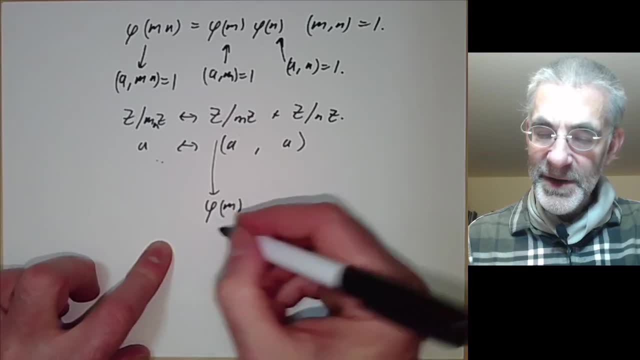 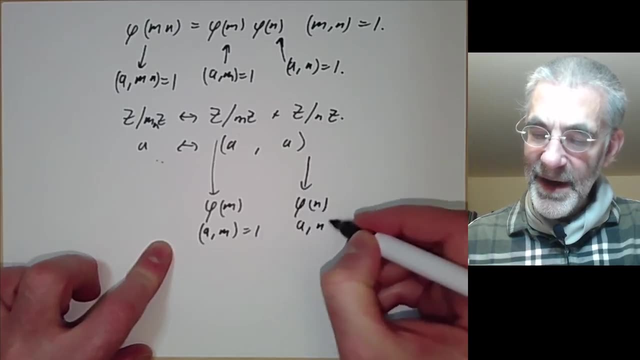 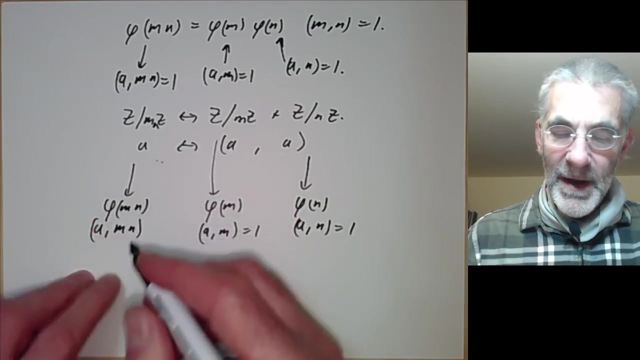 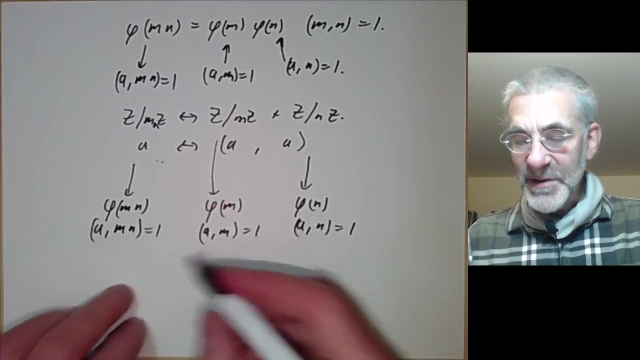 to M. So there are phi M ways of making it coprime and there are phi N ways of making AN equals 1 and there are phi MN ways of making A coprime to MN. And as all these solutions just correspond to any pairs of these two solutions, this: 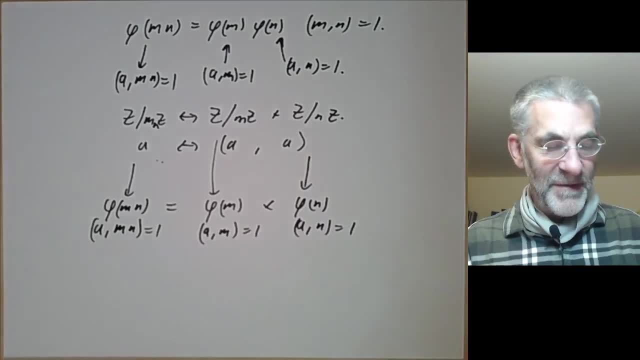 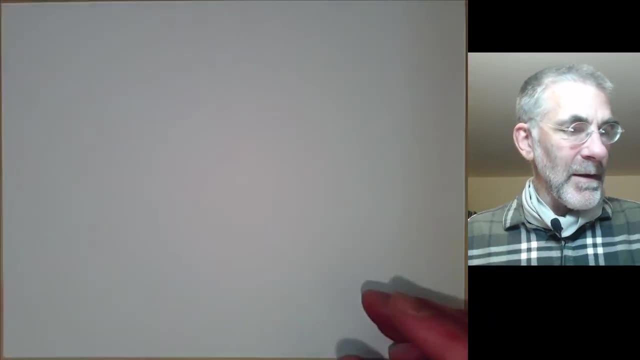 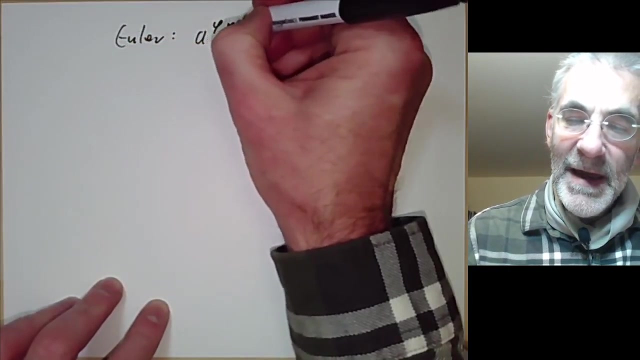 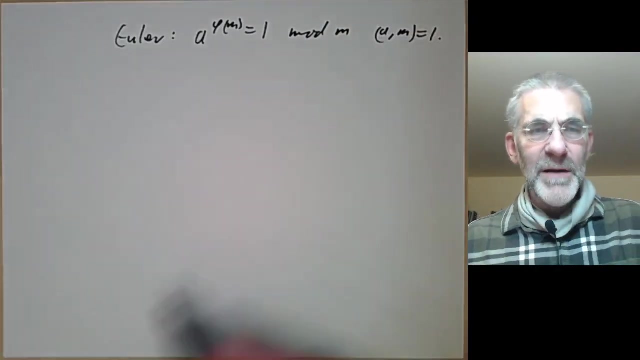 shows that phi of MN is equal to phi of M times phi of N. Next, I mentioned that Euler's theorem says that A to the phi of M is equal to 1 modulo M whenever AM equals 1.. And I mentioned earlier that this was not actually a very good theorem. 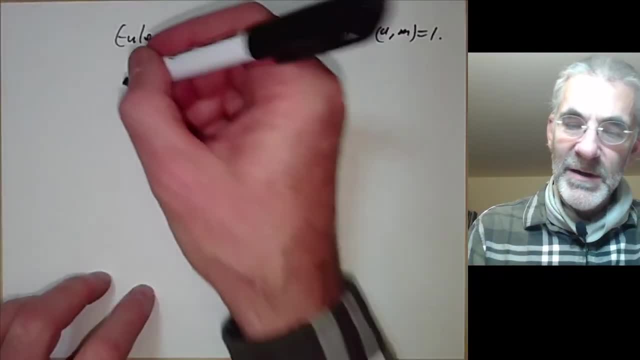 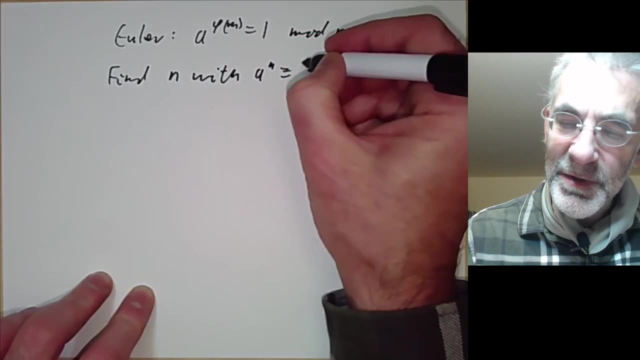 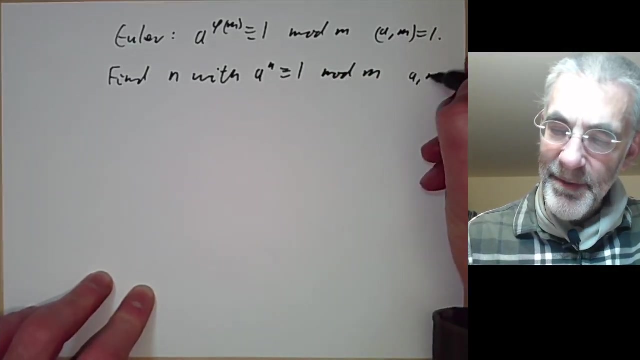 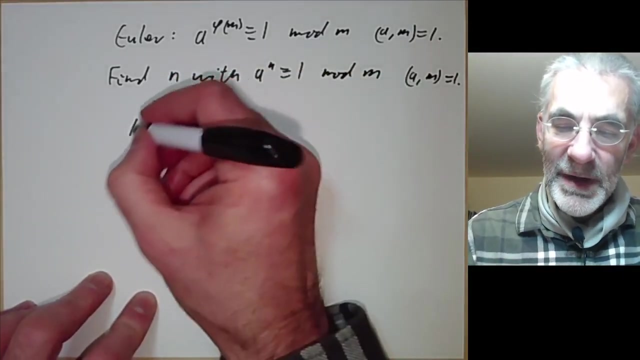 And what I'm going to do now is to try and improve it. So let's find some number N With A to the N is congruent to 1 modulo M for all, A coprime to M, And we can certainly take N equal phi of M. but can we ask: are there smaller values? 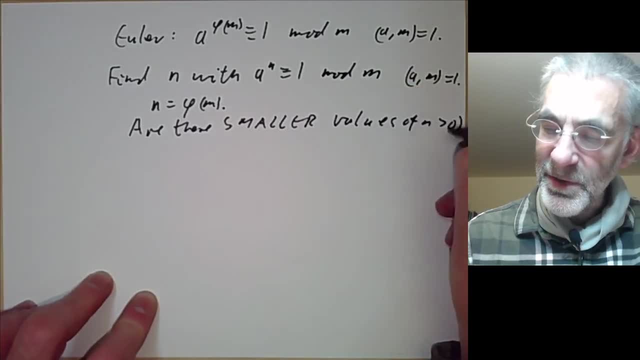 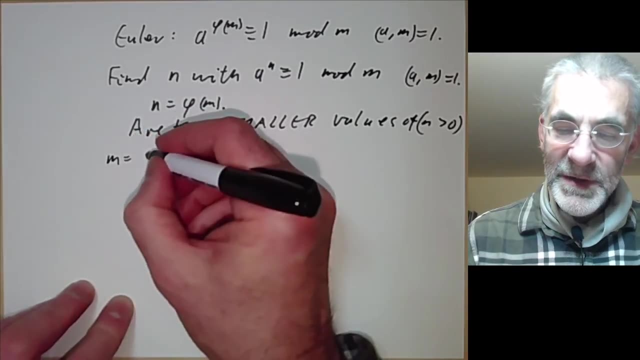 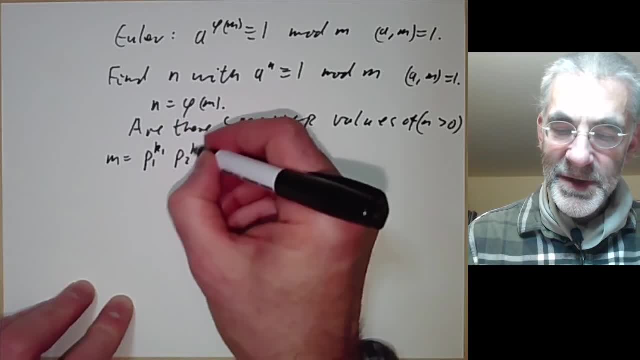 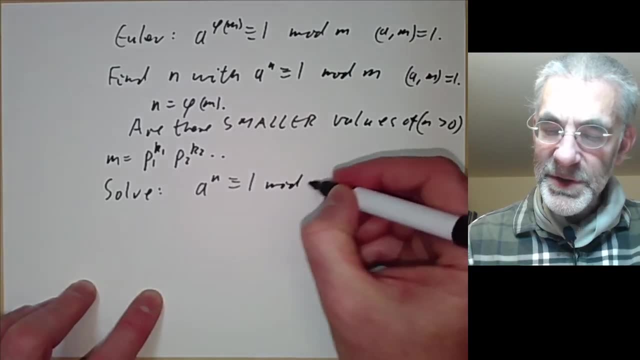 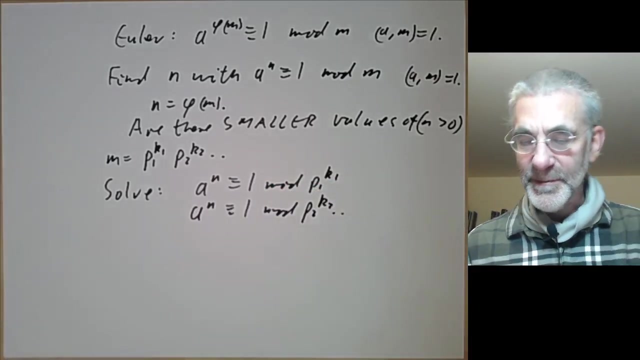 So it's P1 to the K1 times P2 to the K2, and so on. Then we want to solve: A to the N is congruent to 1 modulo, P1 to the K1.. A to the N is congruent to 1 modulo, P2 to the K2, and so on. 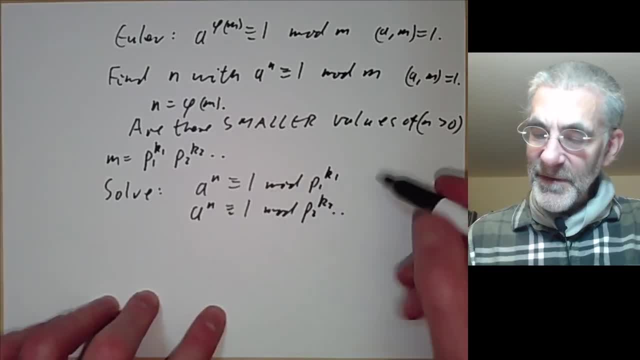 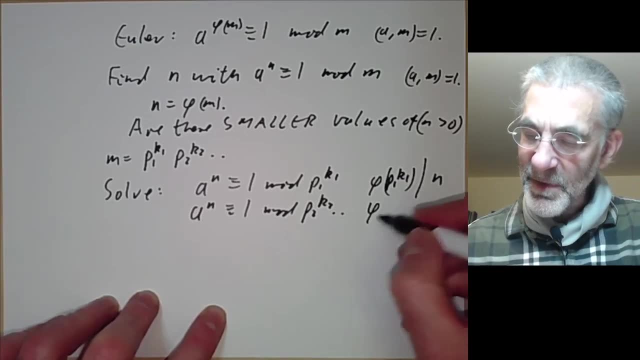 And let's think about this. Well, we can solve this, provided phi of P1 is equal to 1 modulo P2 to the K2.. So phi of P1 to the K1 divides N. And we can solve this: provide phi of P2 to the K2.. 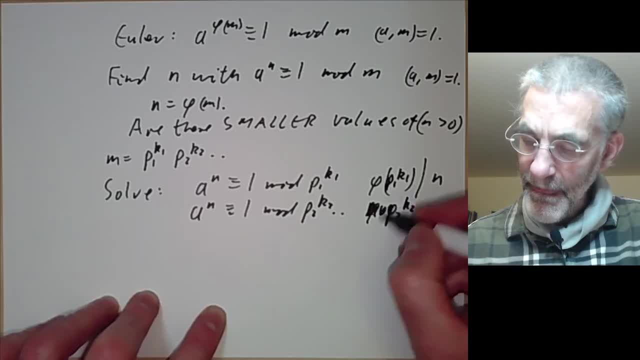 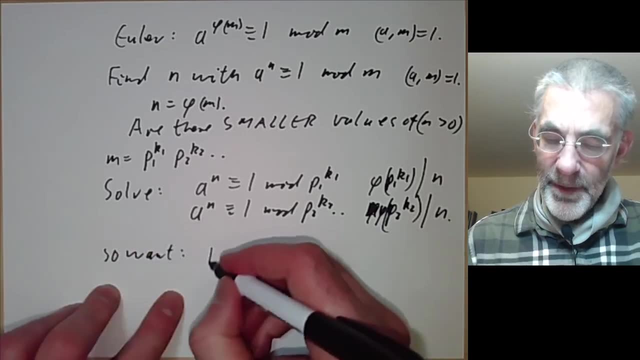 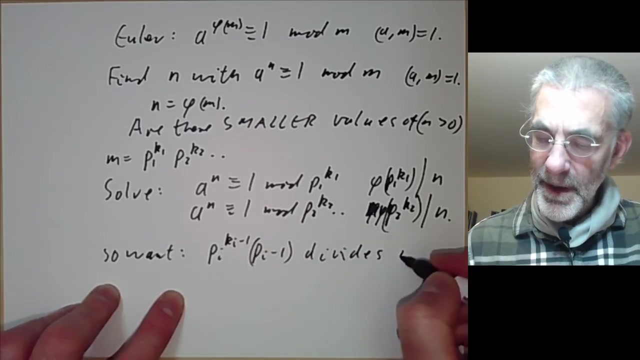 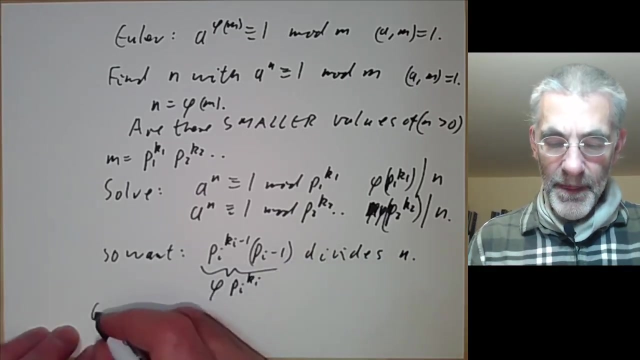 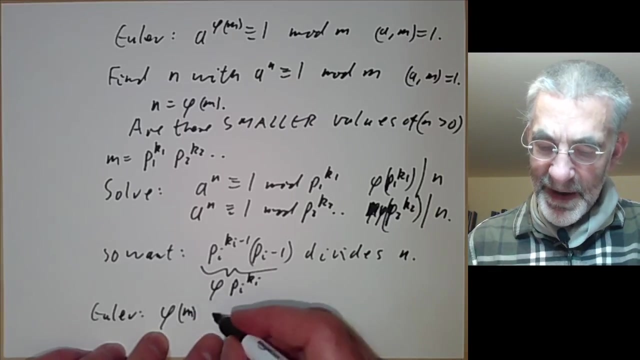 Oops, Sorry, that's a P Divides N. So we want P? i to the K? i minus 1 times P? i minus 1 divides N. So this is, of course, phi of P? i to the K? i And Euler. we just take phi of N, so phi of M, which is the product of these. 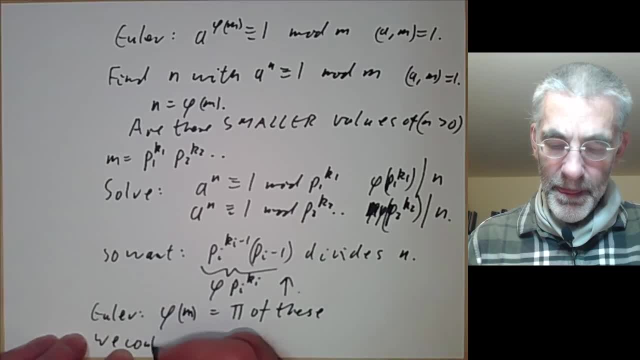 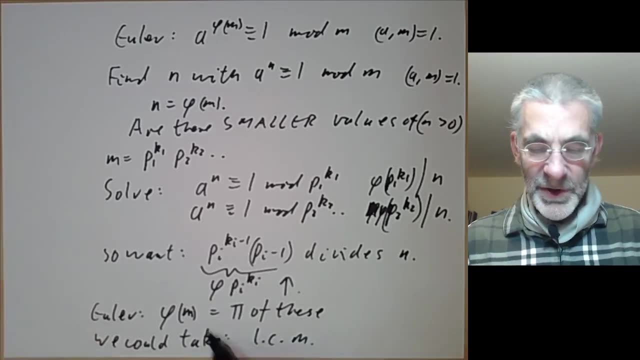 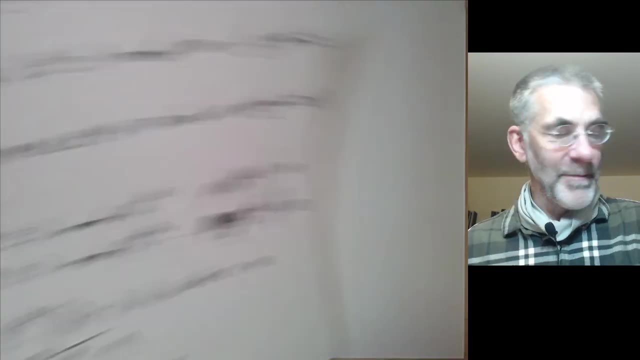 But we don't have to take the product. We could take the least common multiple and this would also do, and it will, in general, be smaller than the product. And this is the product. This is the product. Well, we can do even better than this, because if we look at the prime 2, we know that A 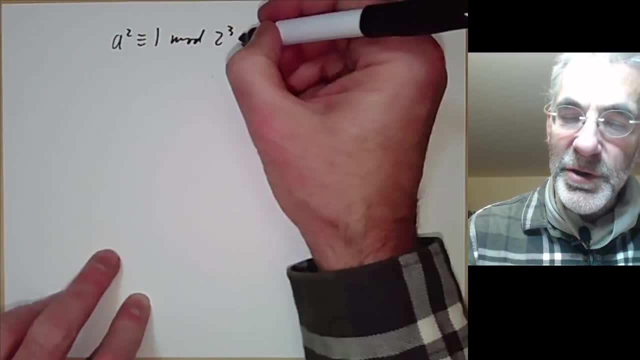 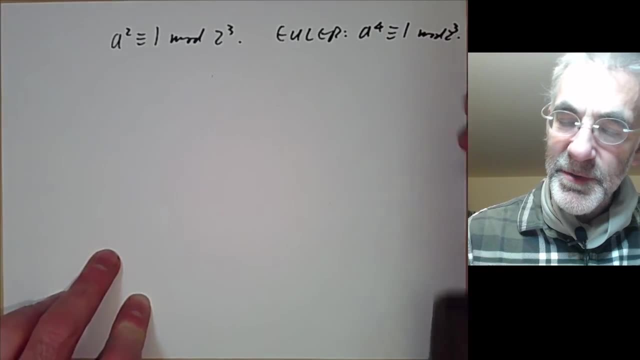 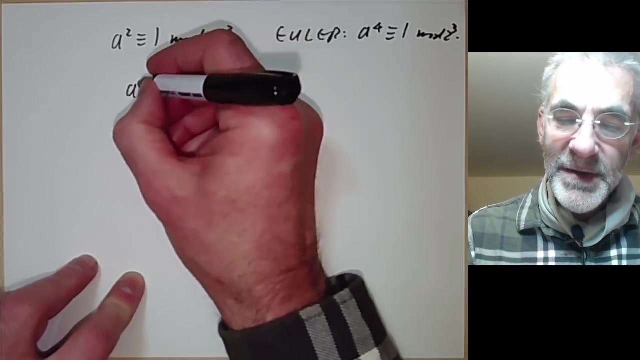 squared is congruent to 1 modulo 2 cubed. But Euler just says that A to the 4 is congruent to 1 modulo 2 cubed And since A squared is congruent to 1 modulo 2 cubed, this easily implies A to the 4 is. 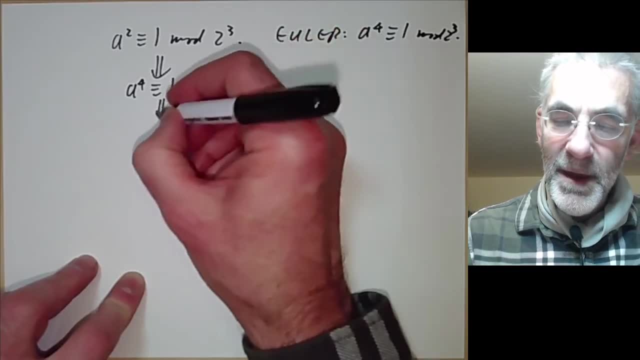 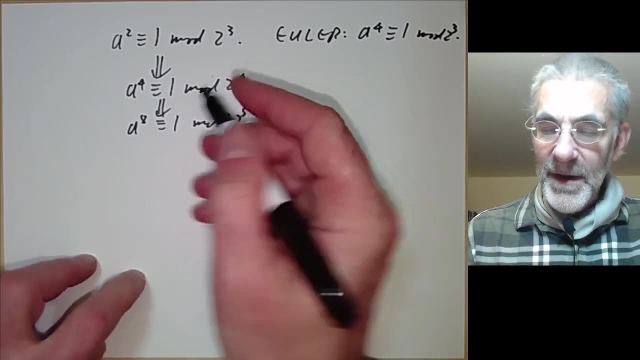 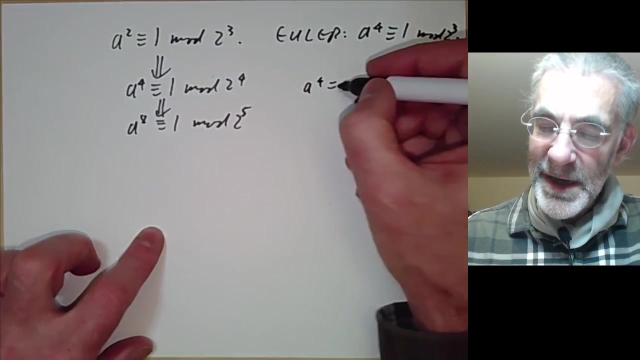 congruent to 1 modulo 2 to the 4.. Which implies A to the 8 is congruent to 1 modulo 2 to the 5 and so on, And you can see this just by repeatedly squaring. For instance, if A to the 4 is equal to 1 plus 2 to the 4 times something, then A to 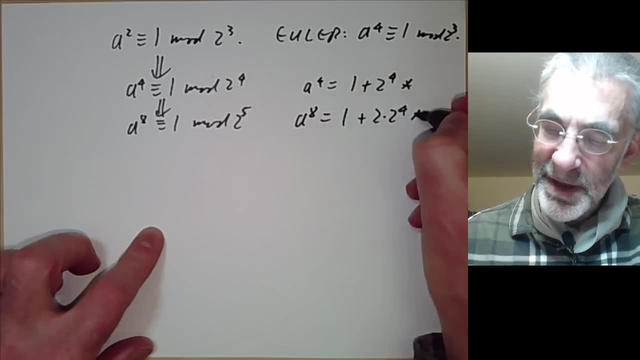 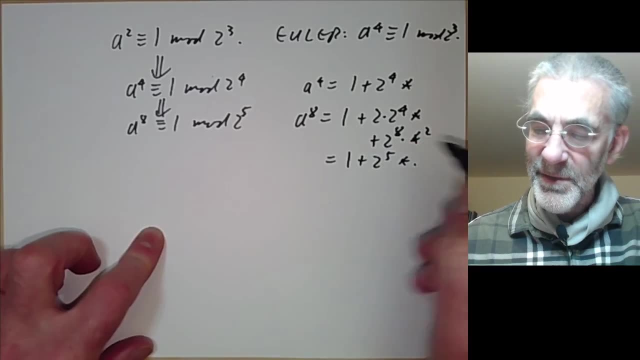 the 8 is going to be 1 plus 2 times 2 to the 4 times something plus 2 to the 8 times something, squared, Which is the form 1 plus 2 to the 5 times something. So in fact we can squeeze out an extra factor of 2.. 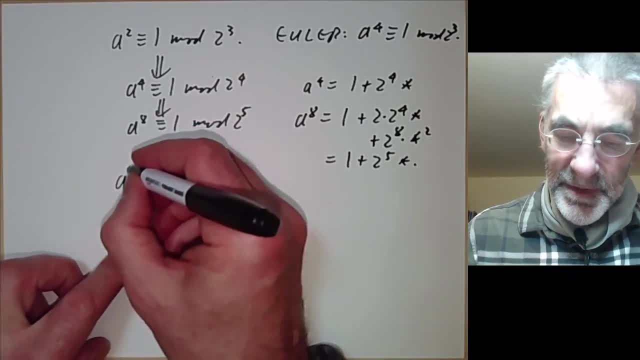 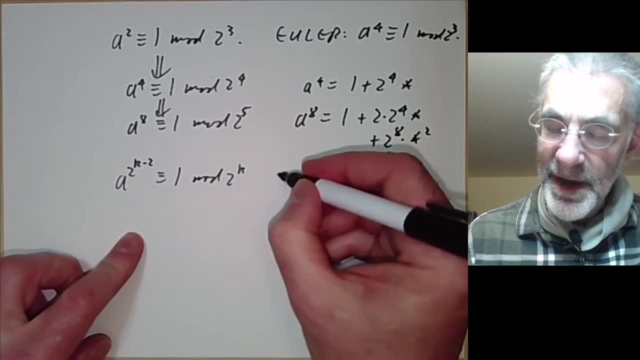 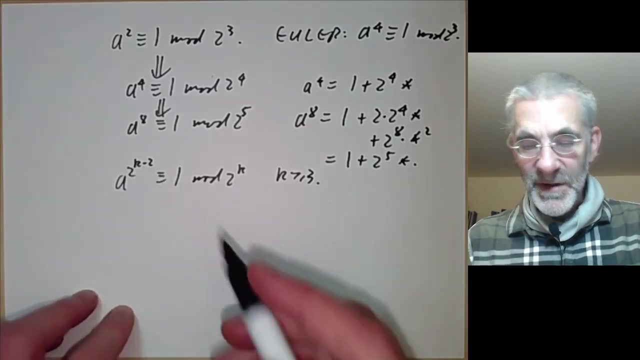 We find that A to the 2 to the k minus 2 is congruent to 1 modulo 2 to the k whenever k is greater than or equal to 3.. And Euler only gives 2 to the k minus 1 instead of 2 to the k minus 2.. 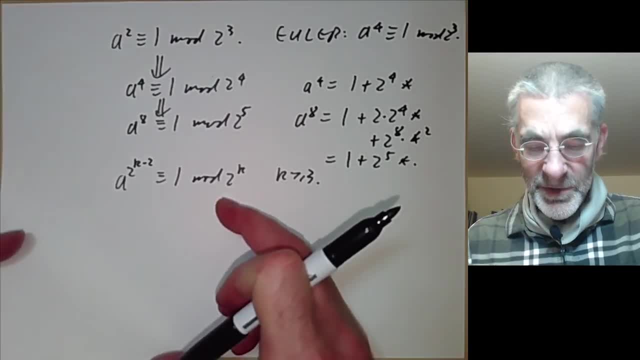 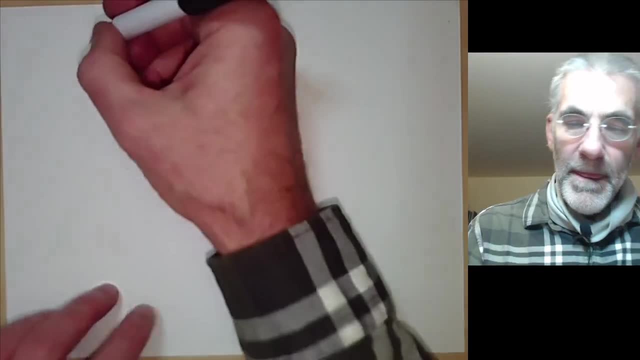 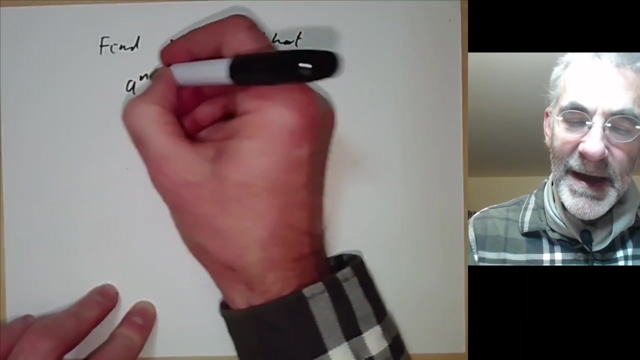 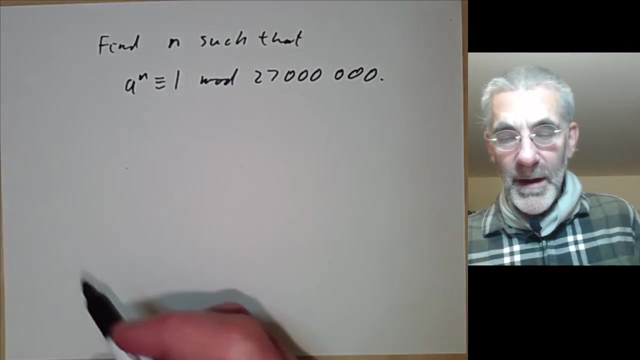 So we can squeeze out an extra factor when the prime is 2.. So let's see an example. Let's find an example of this. Let's find a number n such that A to the n is congruent to 1 modulo 27 million. 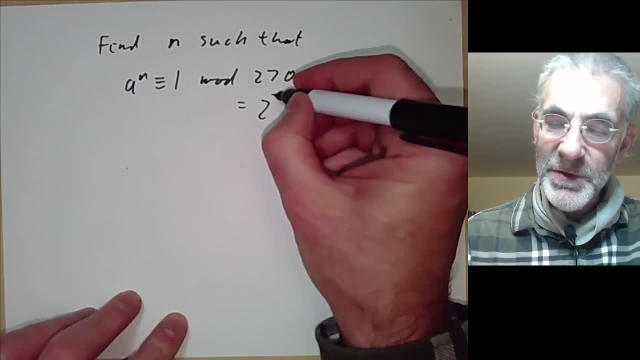 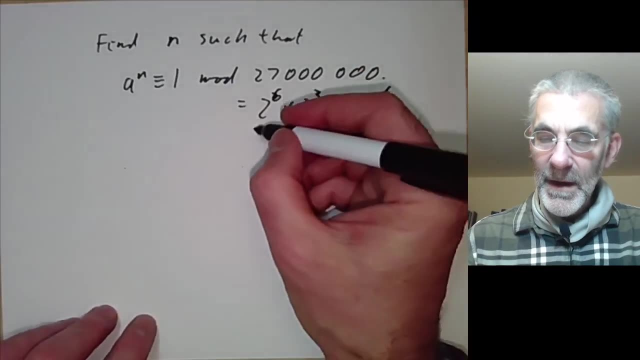 And we first factor this into primes. So this is equal to 2 to the 6 times 3, cubed times 5 to the 6.. And now we work out phi of all these numbers. So phi we get 2 to the 5 here. 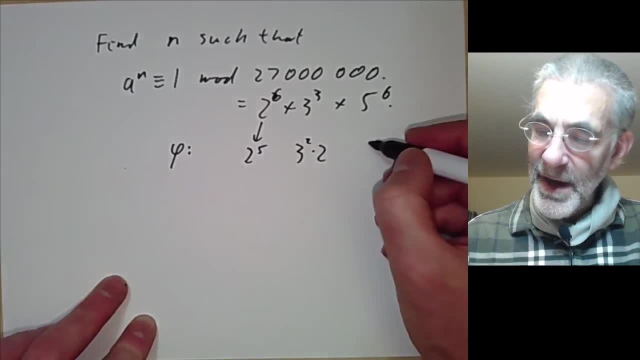 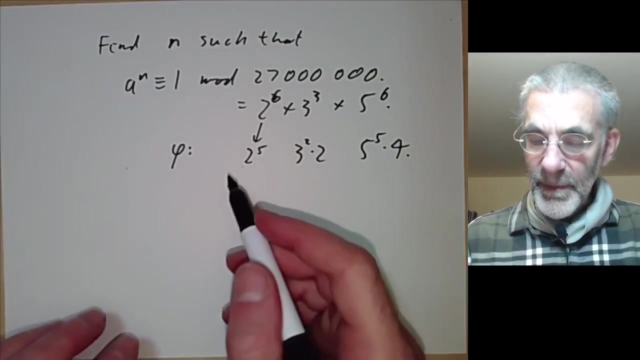 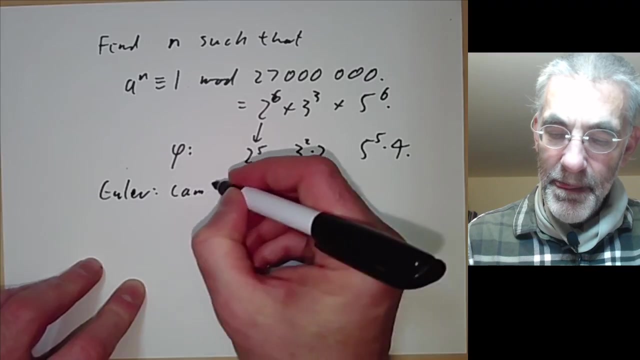 And here we get 3 squared times 2.. And here we get 5 to the 5 times 4.. And now we notice that Euler states: you can take n to be 2 to the 5 times 3 squared times, 2 times 5 to the 5 times 4.. 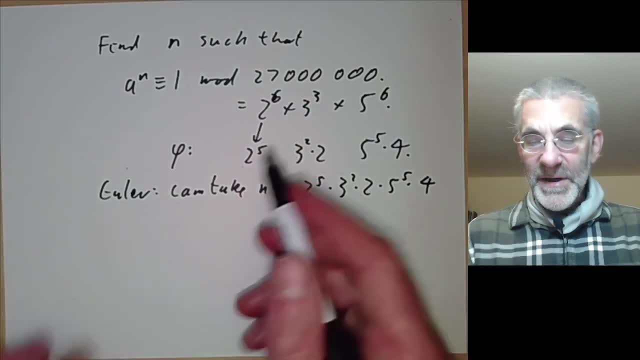 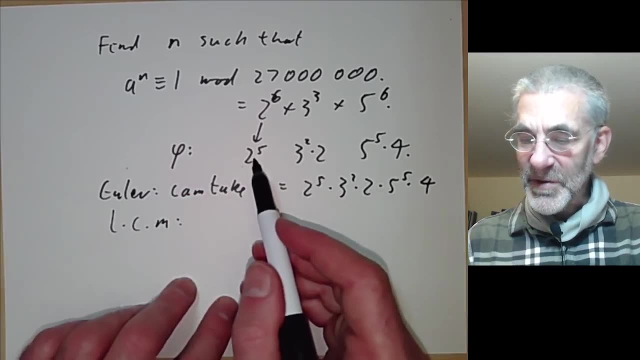 Which is phi of this number here, But instead we can take the least common multiple of these numbers. So we're trying to take the least common multiple of 2 to the 5.. 3 squared times 2 and 5 to the 5.. 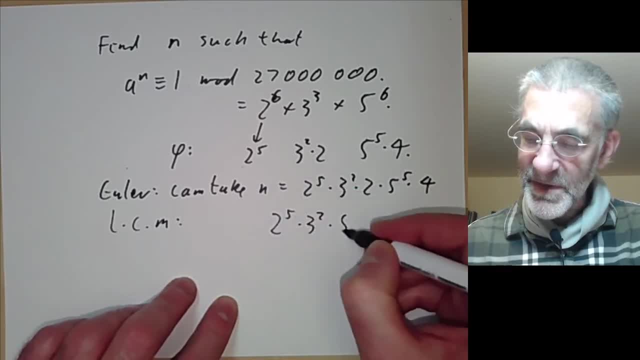 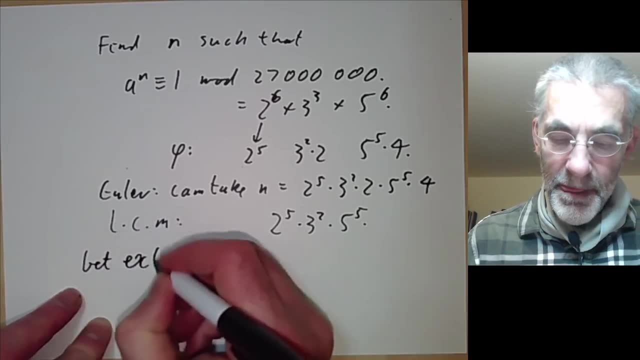 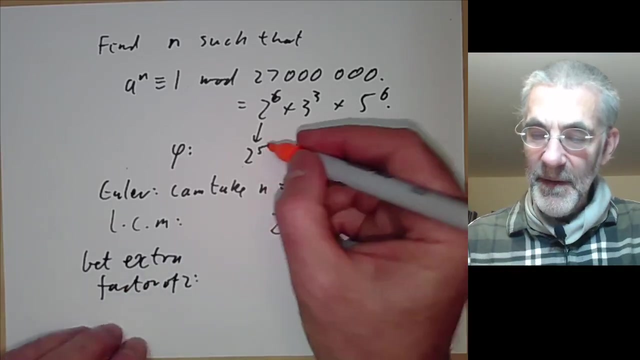 Which gives us 2 to the 5 times 3, squared times 5 to the 5.. But we can do even better. We can get an extra factor of 2.. Because instead of taking 2 to the 5., We can instead use 2 to the 4.. 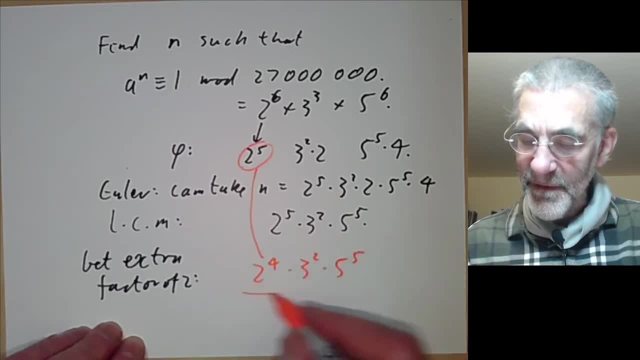 And then of course we've still got the 3 squared times 5 to the 5.. So we can take the least common multiple of 2 to the 5 times 3 squared times 5 to the 5.. And then, of course, we can take n to be this number here. 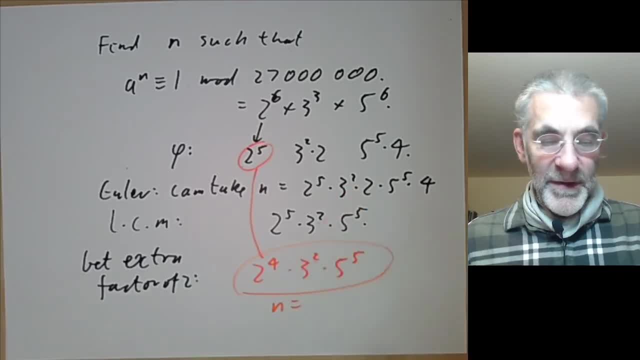 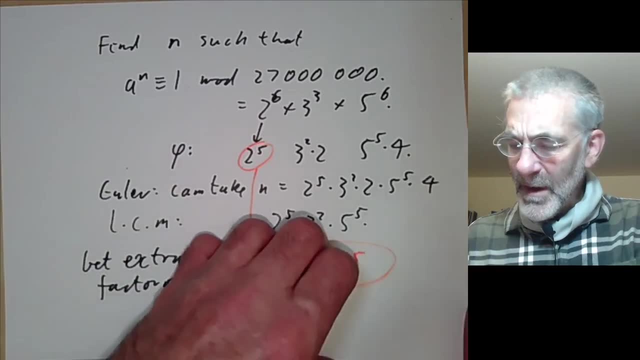 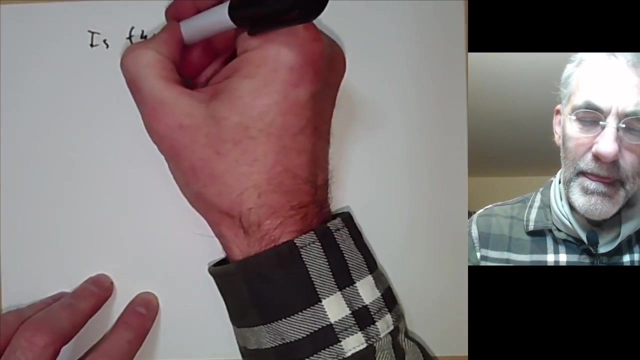 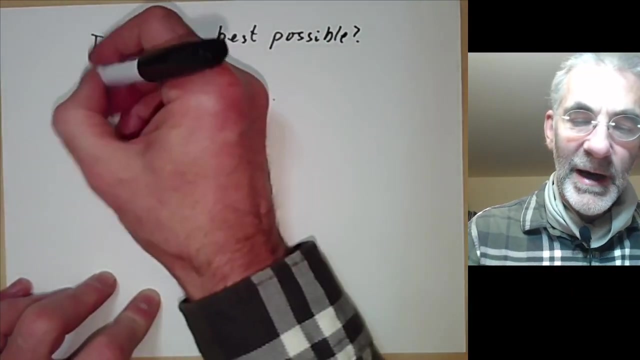 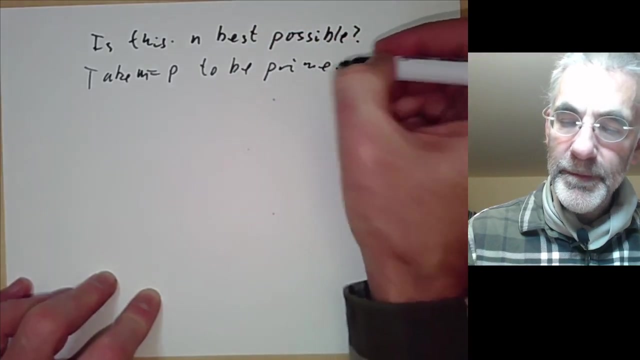 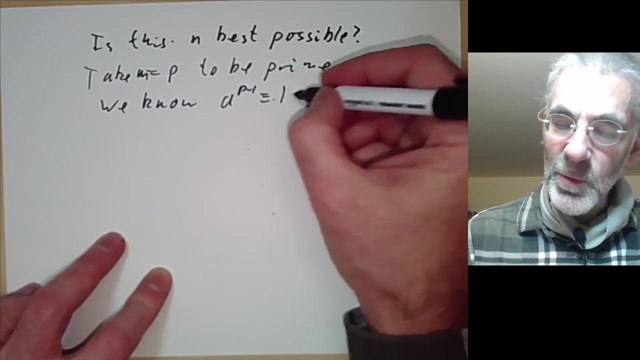 Which is considerably smaller than the number that Euler gives. Now we have the problem: Is the number n we get like this the best possible? In fact, we can ask this for primes. Let's just take m equals p to be prime. Then we know that a to the p minus 1 is congruent to 1 modulo p. 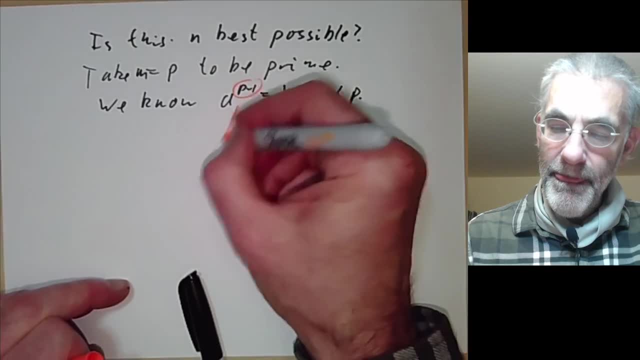 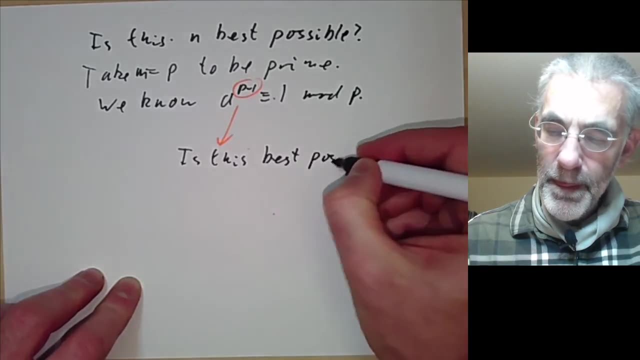 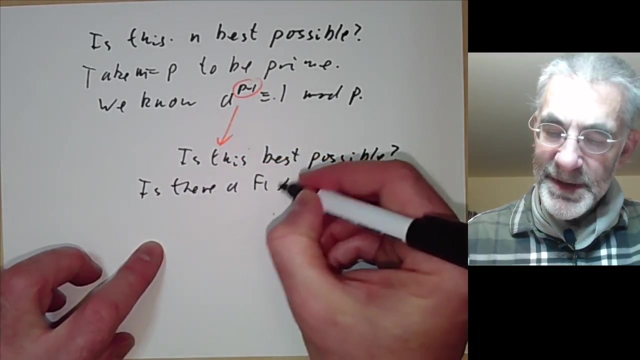 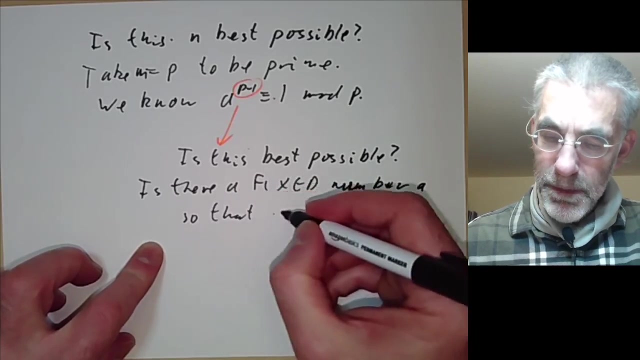 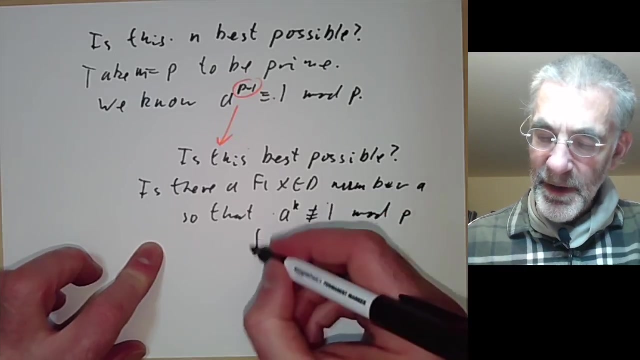 And we ask: can we improve this? So we can ask: is this best possible? And we can ask more generally: is there a number, Is there a fixed number, a, so that a to the k is not congruent to 1 modulo p, for 1 less than or equal to k is less than p minus 1..